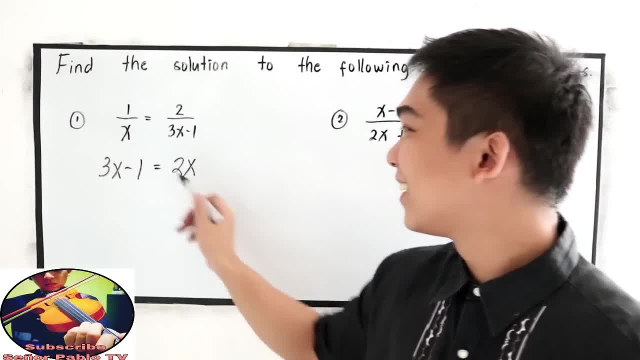 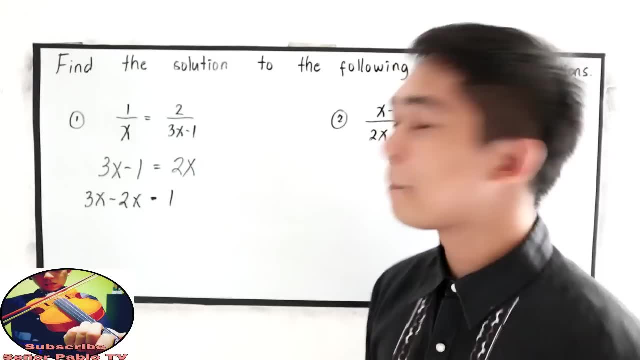 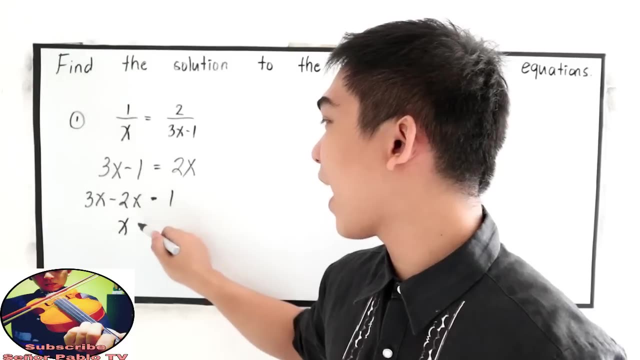 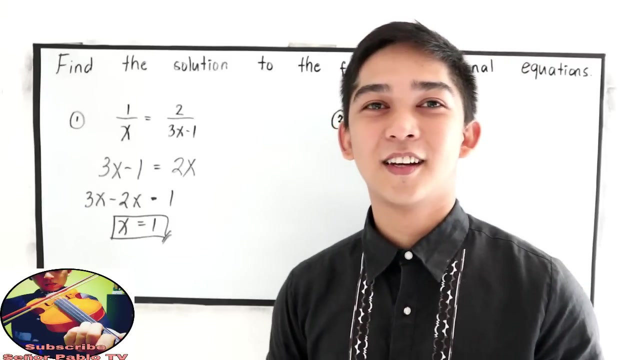 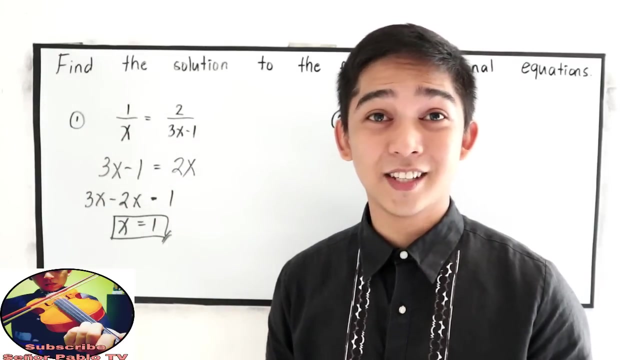 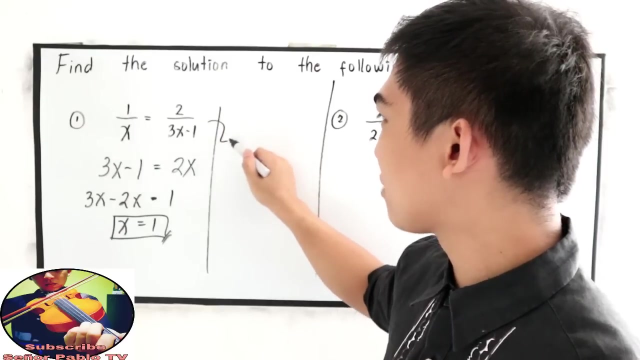 Now combine like terms, Sorry. So 3x minus 2x is equal to positive 1.. Next, 3x minus 2x, That is x is equal to 1.. Okay, The other way is using the or getting the LCD. Let's say: okay, the other way is: I will write my solution here. 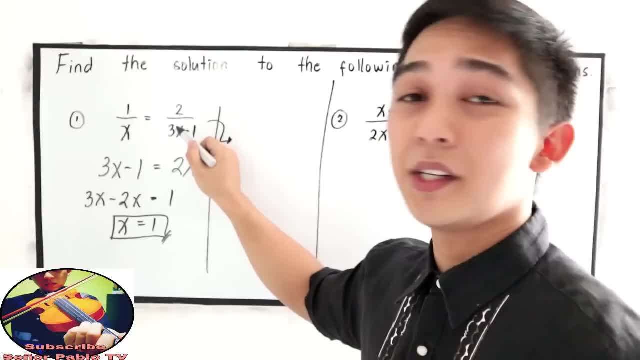 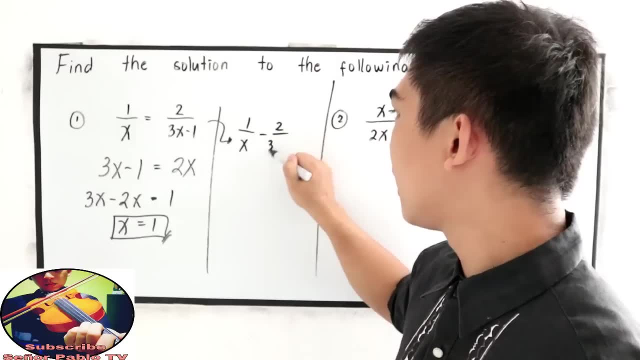 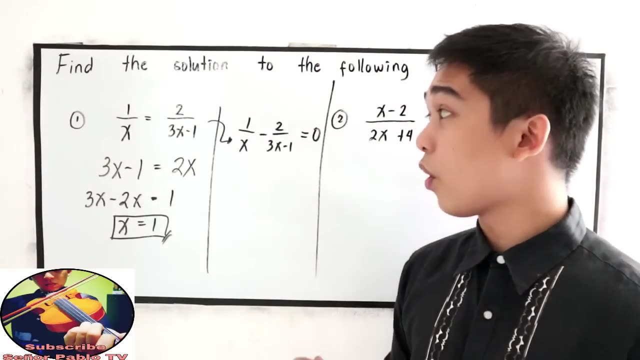 So I'm going to transpose 2 over 3x 3x minus 1.. So that will become 1 over x minus 2 over 3x minus 1 is equal to 0.. We transpose 2 over 3x minus 1.. 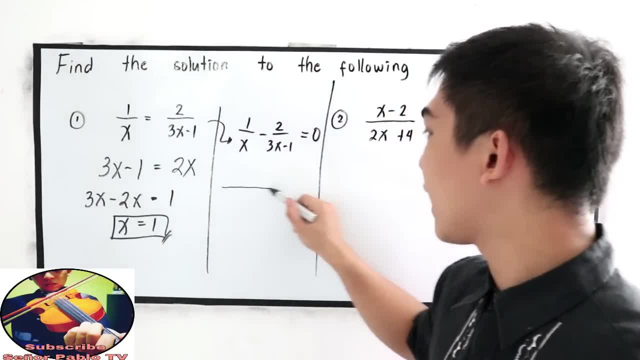 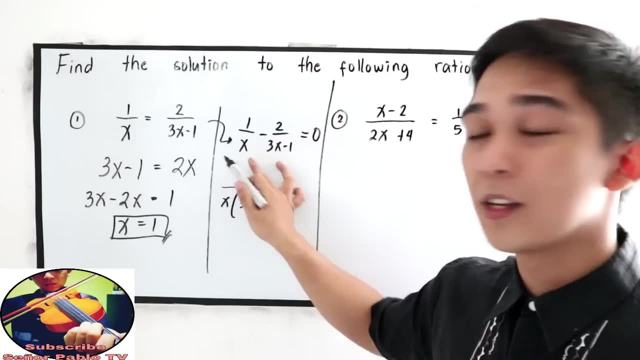 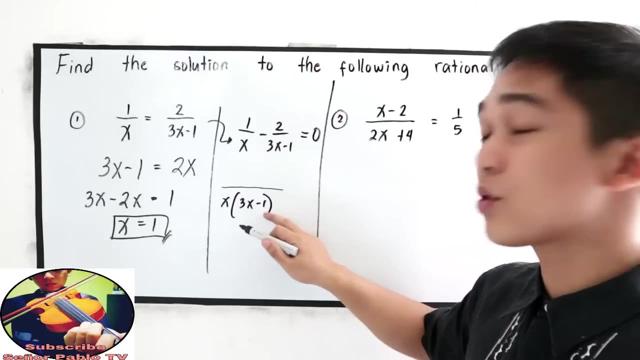 Now find the LCD. Our LCD is x times 3x minus 1.. Our denominator So x times 3x minus 1.. Divided by x, That is 3x minus 1 times 1. 3x minus 1.. 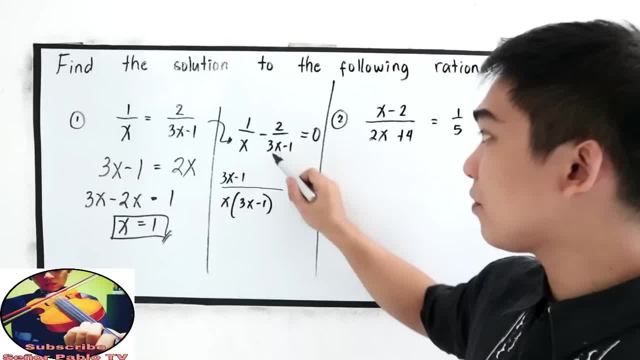 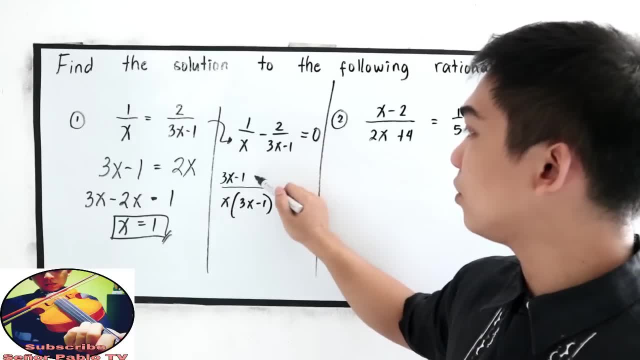 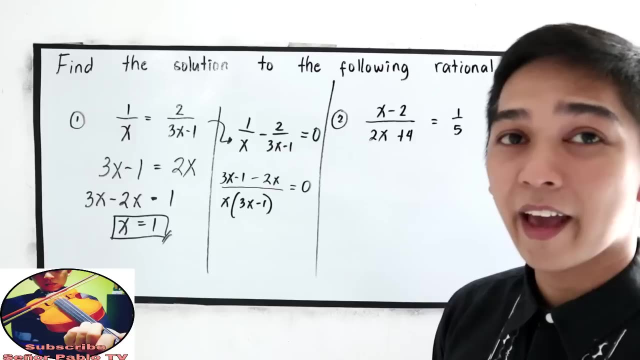 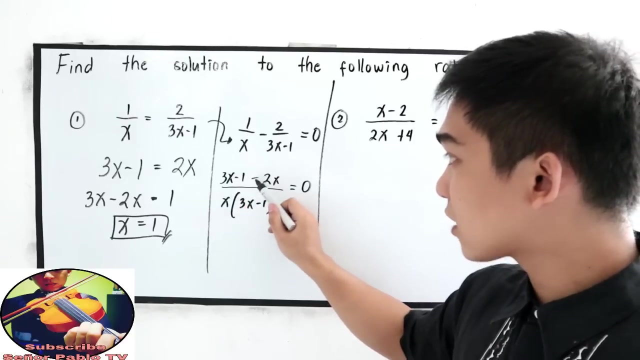 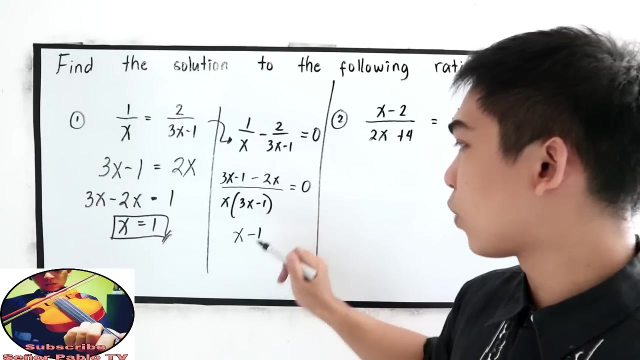 Next: x times 3x minus 1 divided by 3x minus 1.. That is x multiplied by 2.. Negative 2x is equal to 0.. And next combine like terms in our numerator: 3x minus 2x, That is x. then copy minus 1 over: x times 3x minus 1 is equal to 0. 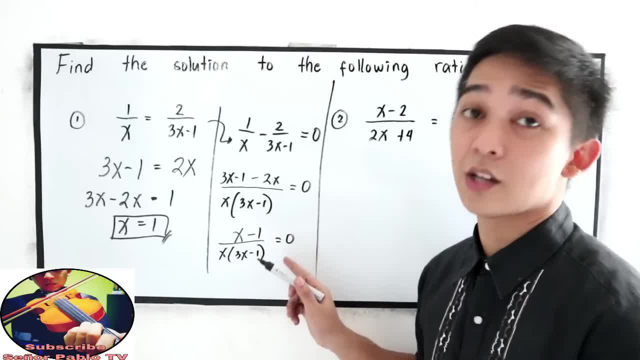 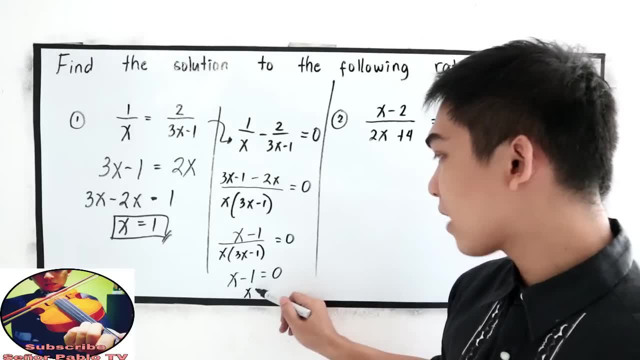 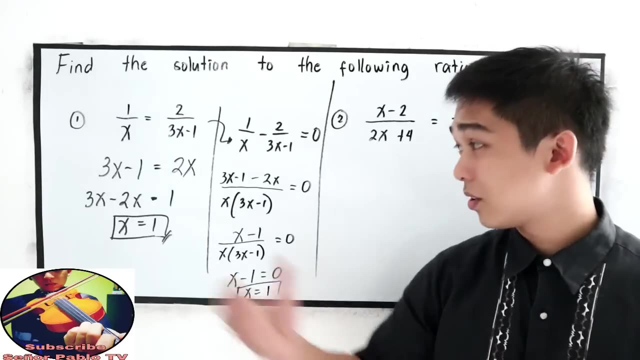 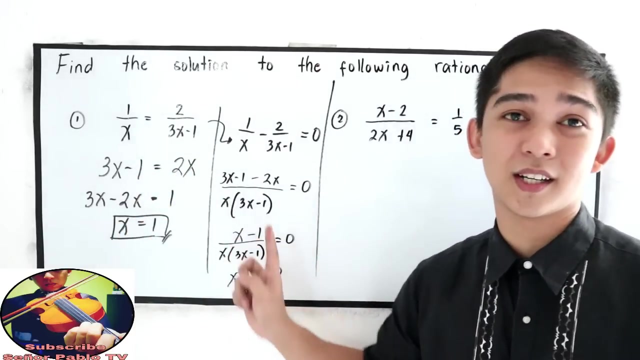 Now our denominator multiplied to 0. That is to become 0. So next will be: x minus 1 is equal to 0. And now x is equal to positive 1, which is the same. So you will choose which method you're going to use. You can use the easier one or the moderate one. 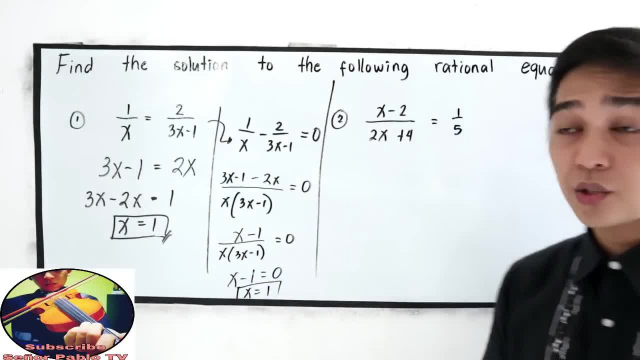 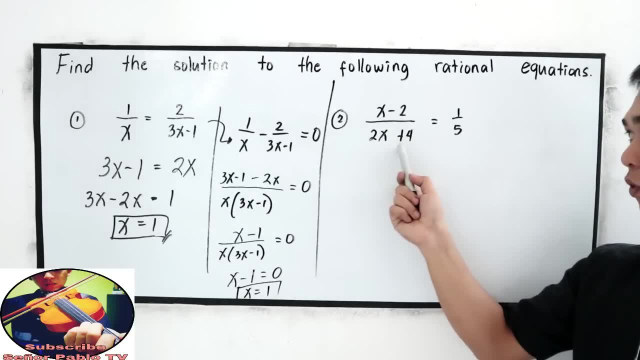 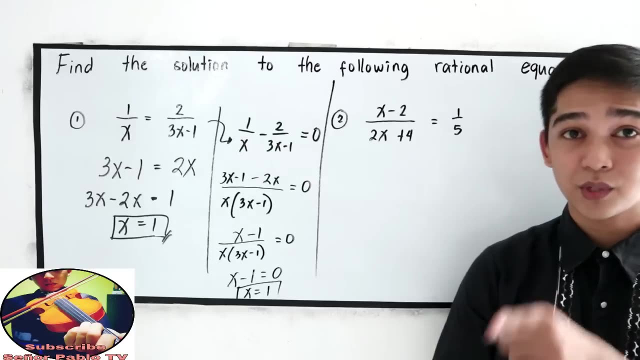 Now I want you to try number 2.. x minus 2 all over 2x plus 4 is equal to 1.. x minus 2 all over 2x plus 4 is equal to 1 over 5.. If you want to try, you can pause the video. 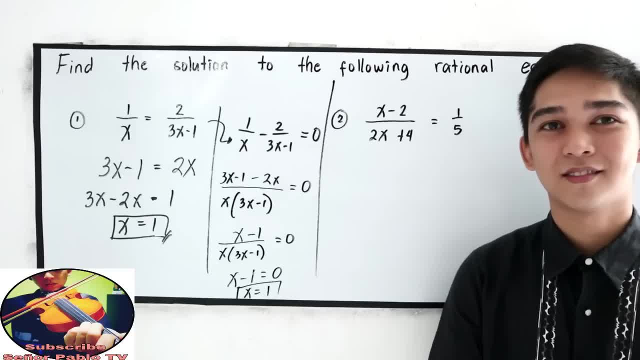 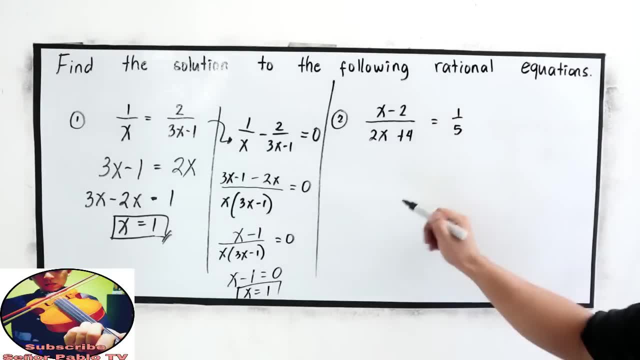 And, after answering, resume watching. Okay, let's try. Let's use the easiest way: Cross multiply, that will become 5 times x minus 2.. Next, 2x plus 4 times 1, that will become 2x plus 4.. 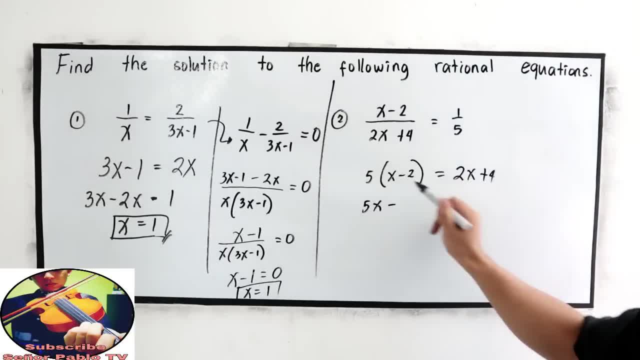 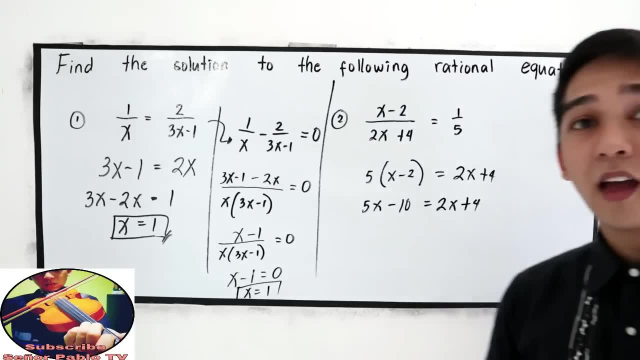 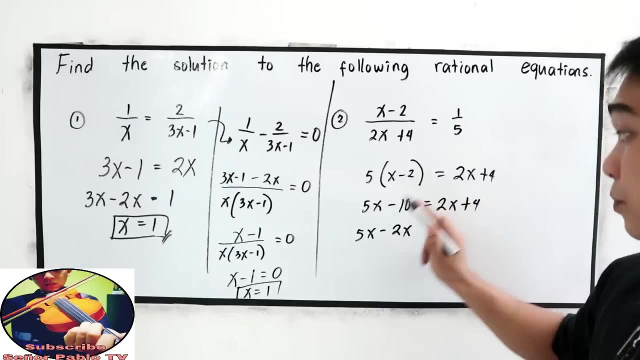 Distribute: 5x minus 10 is equal to 2x plus 1.. And now combine like terms: 5x minus 2x. we transpose 2, is equal to 4.. 4 plus 10.. 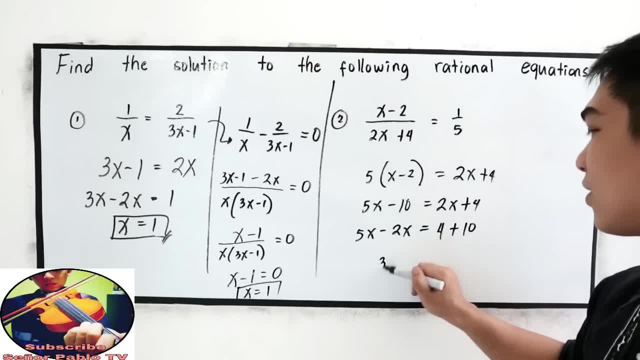 5x minus 2x, that is 3x, is equal to 14.. And now to get x, we need to divide by 3.. Divide it by 3.. So x is equal to 14 over 3.. 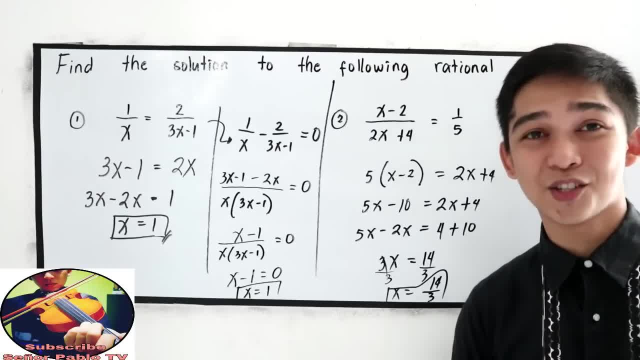 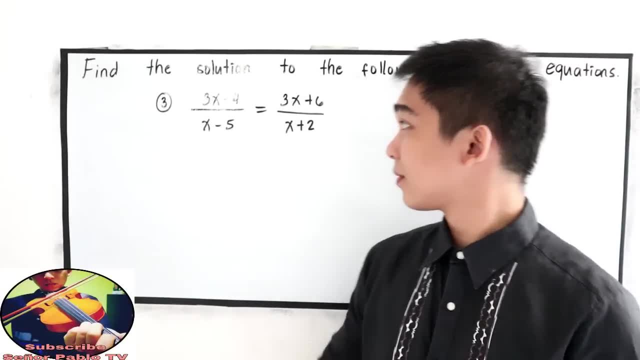 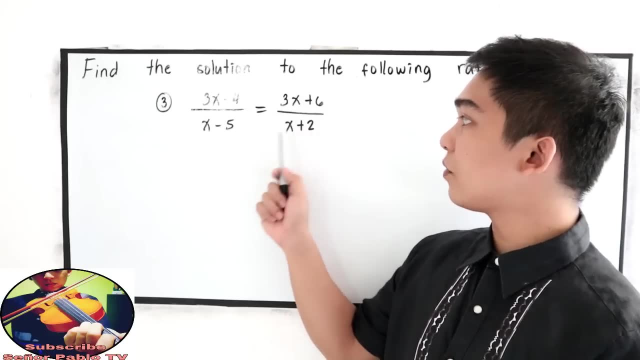 14 over 3 will be our final answer. Did you get the same answer? Now let's try number 3.. 3x minus 4 over x minus 5 is equal to 3x plus 6, all over x plus 2.. 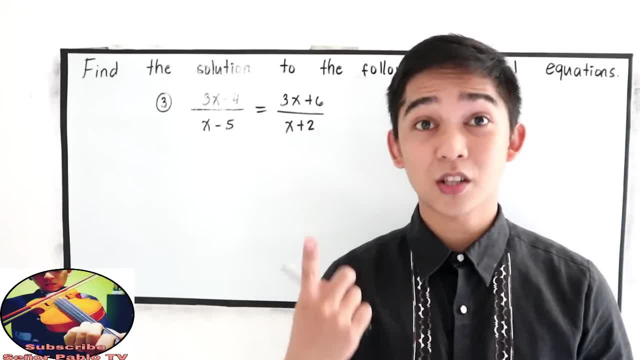 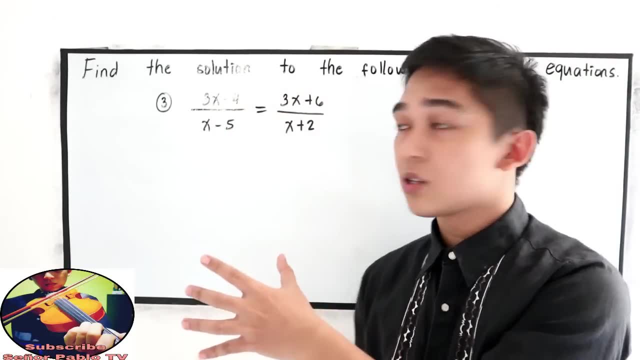 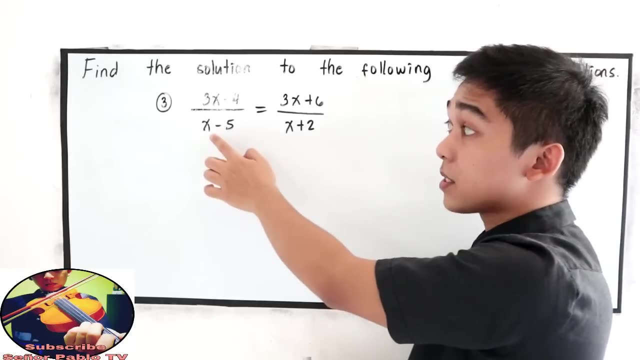 So our first step, we need to cross multiply, But before doing our equation. so look at our denominator, Our domain or the value, Because for x it must not be equal to 5 on the left side of the equation. 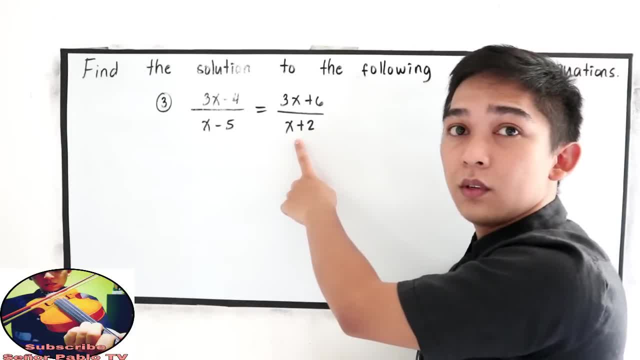 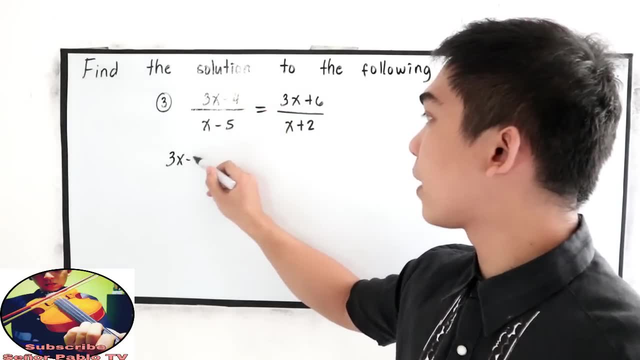 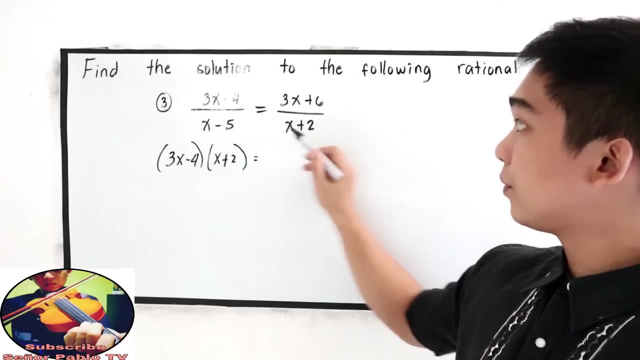 And on the right side, x must not be equal to 2. Because that will give us undefined So cross. multiply That will become 3x minus 4 times x plus 2 is equal to 3x plus 6 times x. 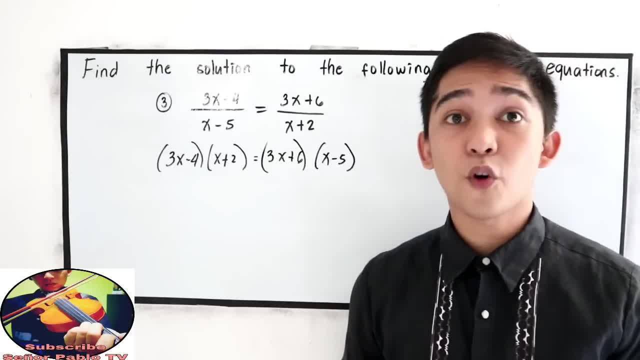 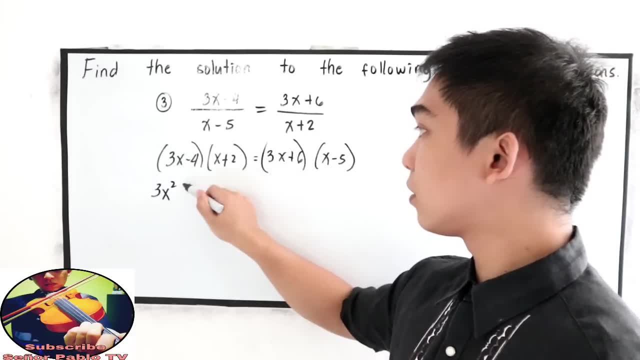 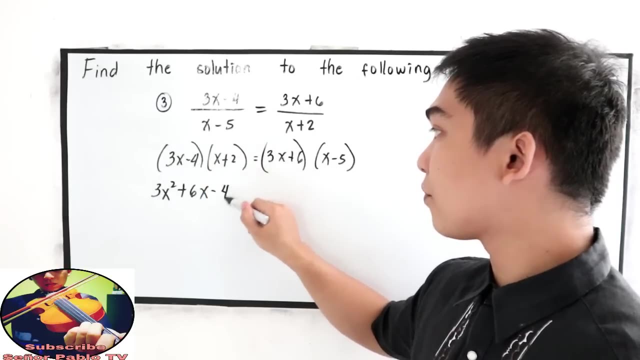 3x minus 5.. Then use the FOIL method. So 3x times x, 3x squared, 3x times 2, positive 6x. Next negative 4 times x, negative 4x. 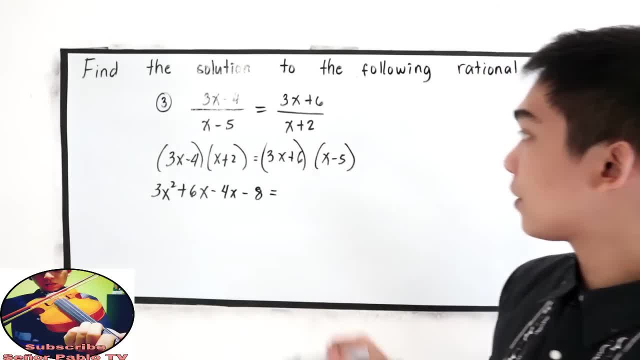 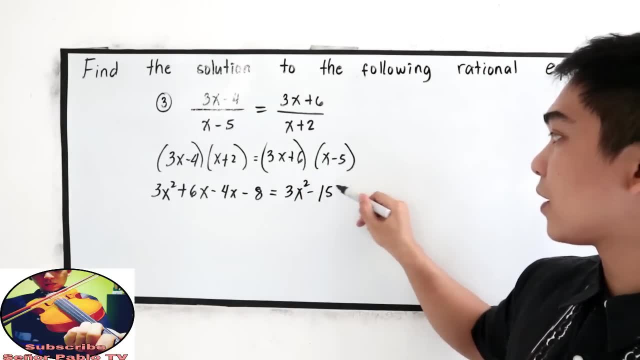 Negative 4 times 2, negative 3. Is equal to 3x times x, 3x squared. 3x times negative: 5, negative, 15x. 6 times x, positive, 6x. Then 6 times negative, 5, negative 15.. 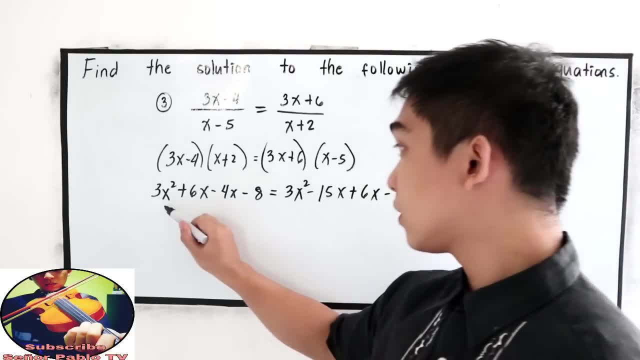 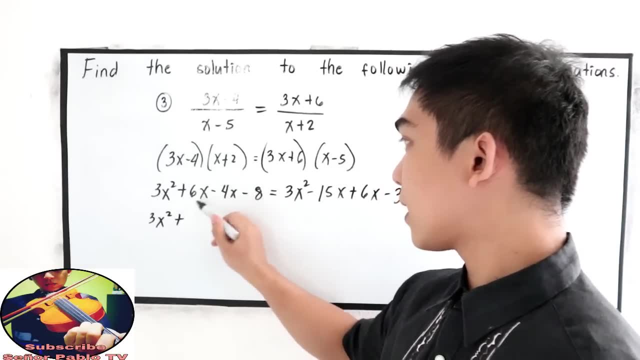 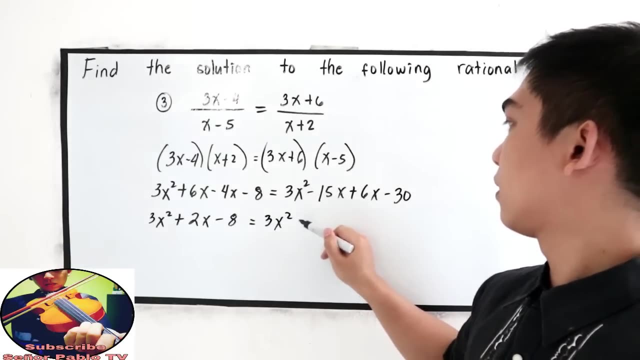 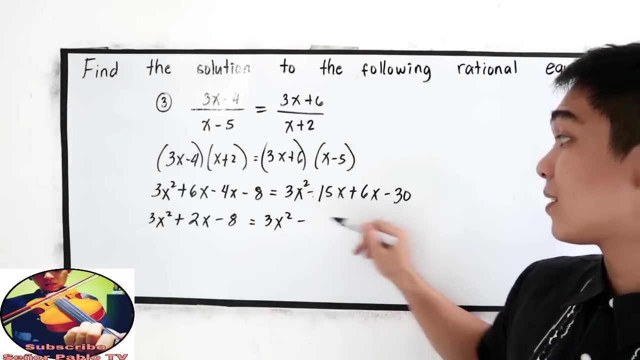 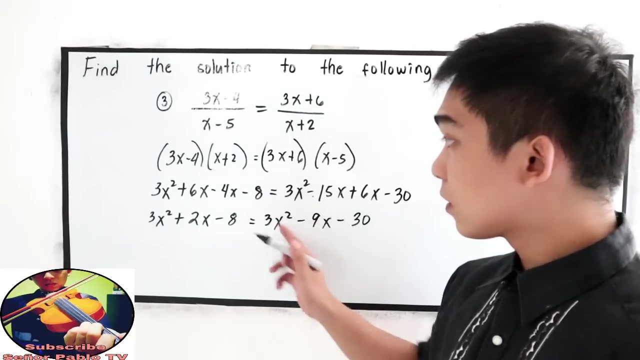 Now combine like terms, This will become: 3x squared plus 2x minus 8 is equal to 3x squared negative 15x plus 6x. This is negative 9x minus 30.. And combine like terms: 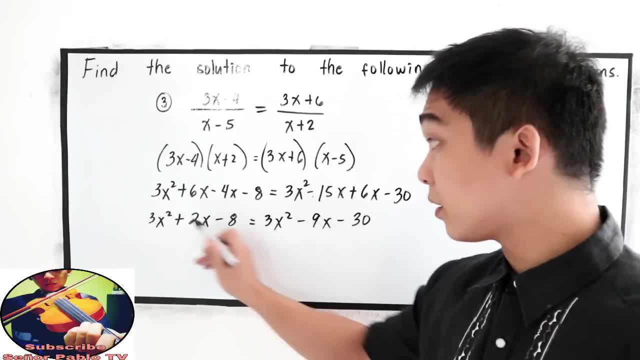 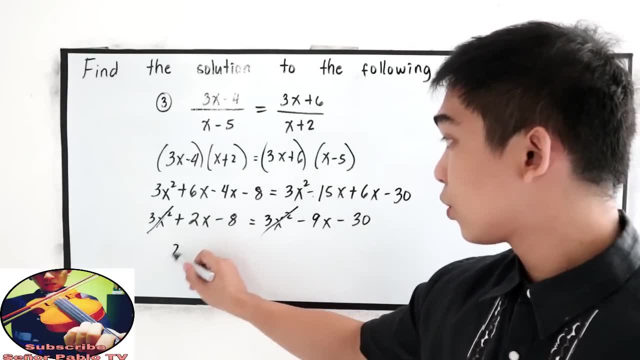 Notice that if we're going to transpose 3x squared, this will be 0. So we can cancel that out. Then 2x plus 9x is equal to negative 30. transpose negative 30.. So we can cancel that out. 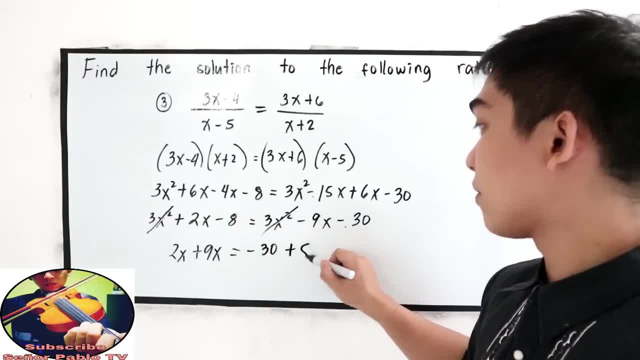 Then 2x plus 9x is equal to negative 30. transpose negative 30.. Then 2x plus 9x is equal to negative 30. transpose negative 30.. Suppose negative 8, that will become a positive 8.. 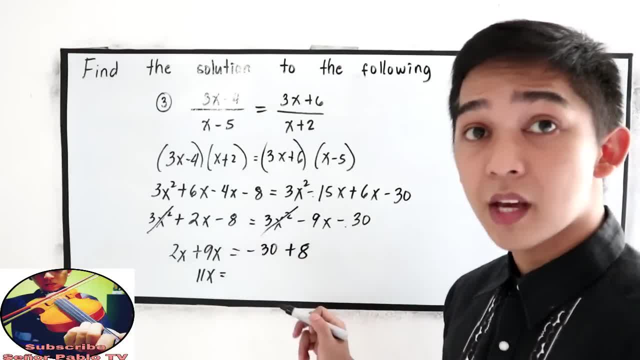 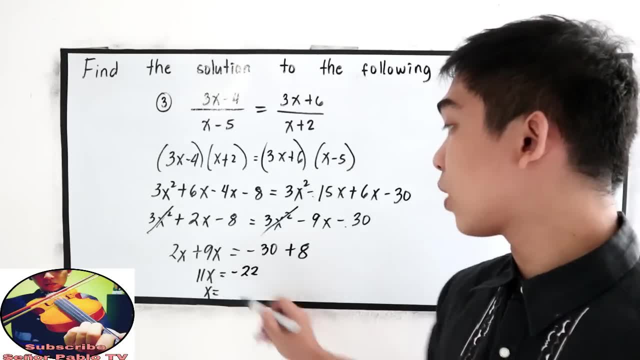 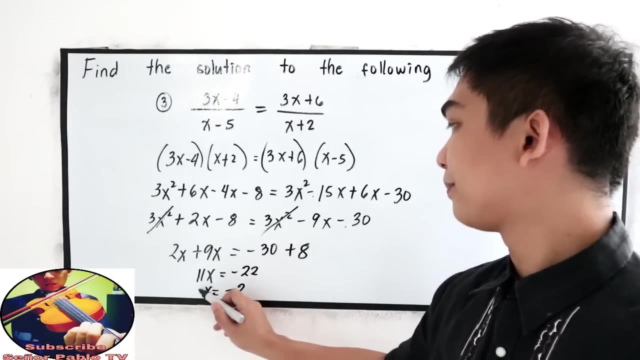 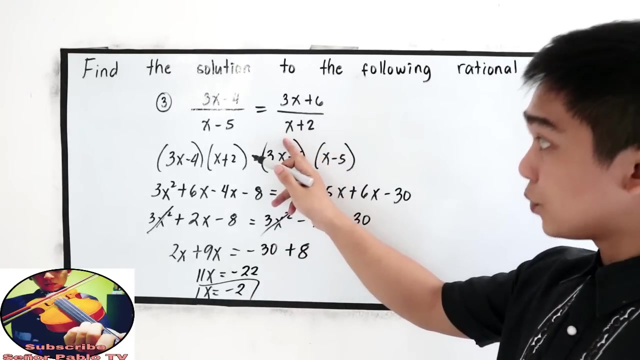 So 11x is equal to negative 30 plus 8, negative 22.. Get the value for x. So x is equal to negative 22 divided by 11. So negative 2.. If we're going to substitute negative 2.. 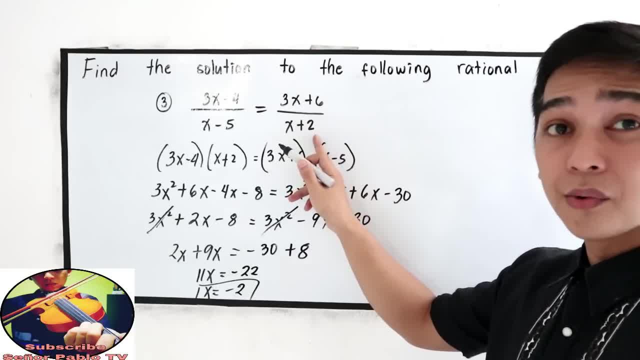 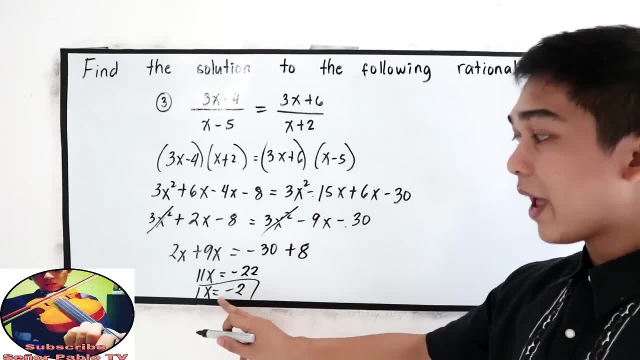 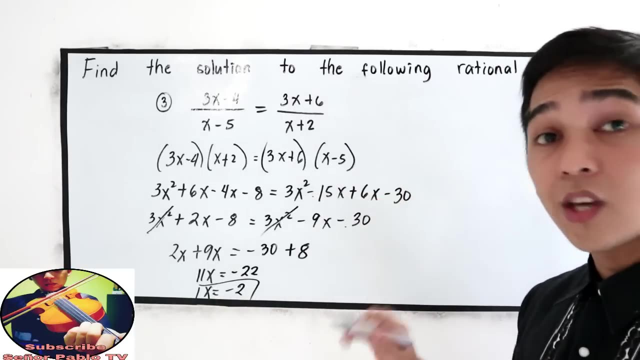 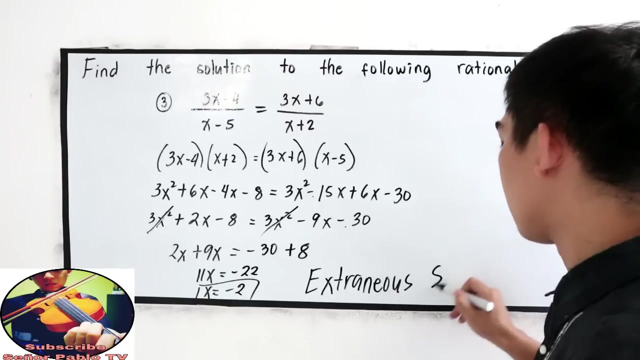 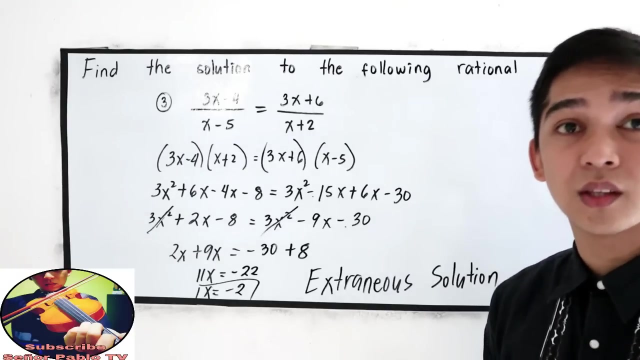 Plus 2, that will become 0, which is not applicable because it will give us undefined. So the value of x is not applicable. So we call this equation as x. it has extraneous solution If the value of x or if our solution will make our equation undefined. 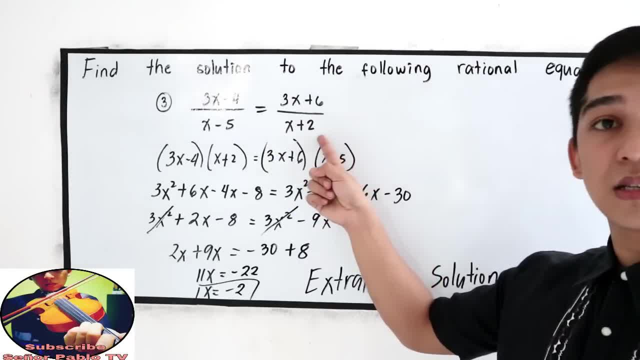 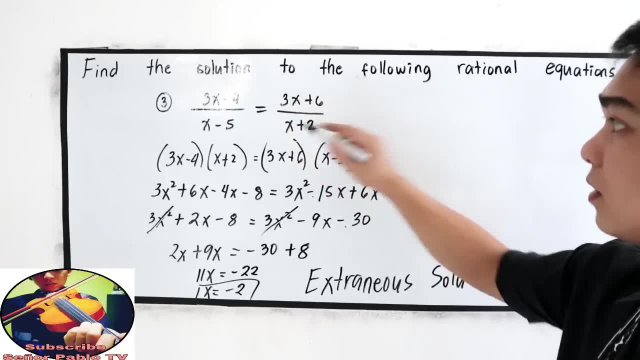 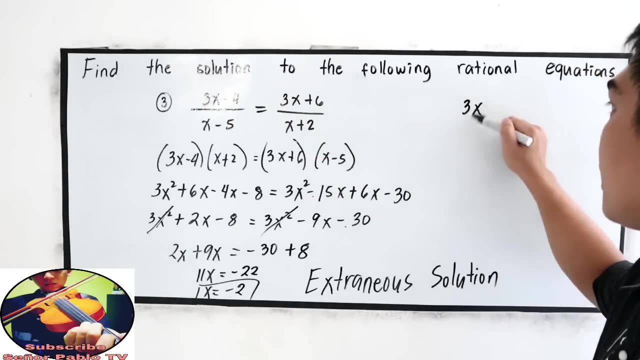 There is another way to solve this rational equation. Take a look at our equation on the right side, that this will be, or this can be cancelled out, So So copy the left side of the equation: 3x-4 all over x-5 is equal to let us factor the numerator. 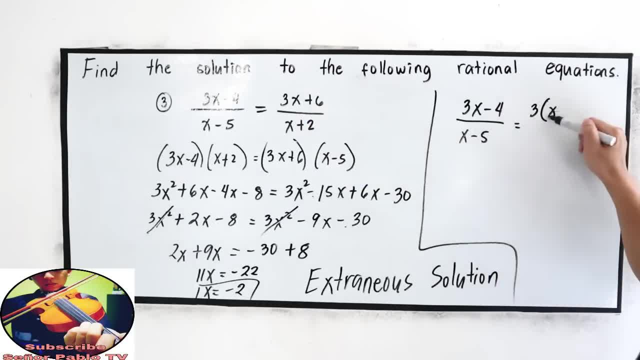 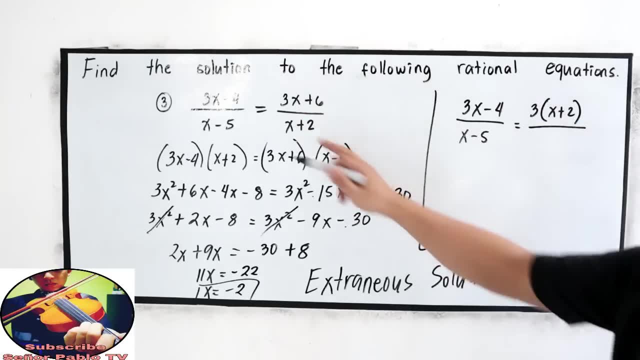 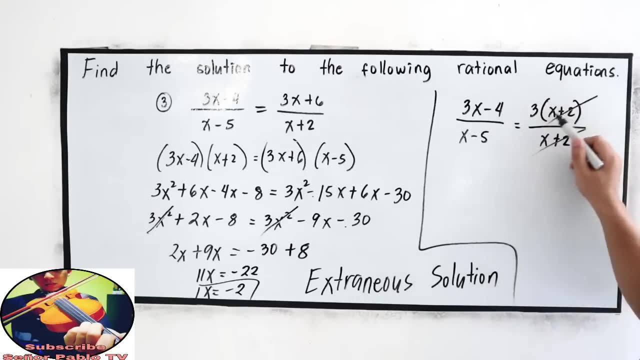 That is x3 times x plus 2,, 3 times x, 3x, 3 times 2, negative positive 6, over x plus 2.. Now we can cancel, So we have x plus 2, and x plus 2.. 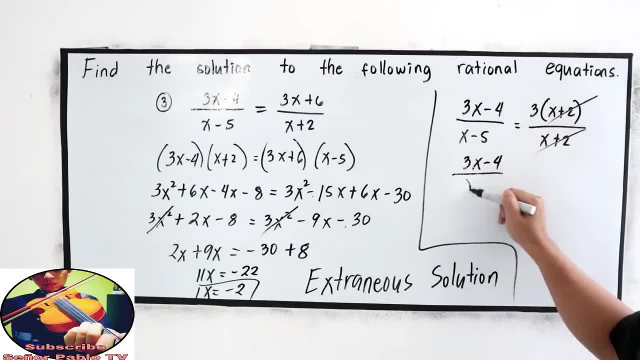 The remaining is 3x-4 all over. x-5 is equal to: then cross multiply So we have: 3x-4 is equal to 3 times x, 3x negative, 3 times negative, 5 times 3, negative 15.. 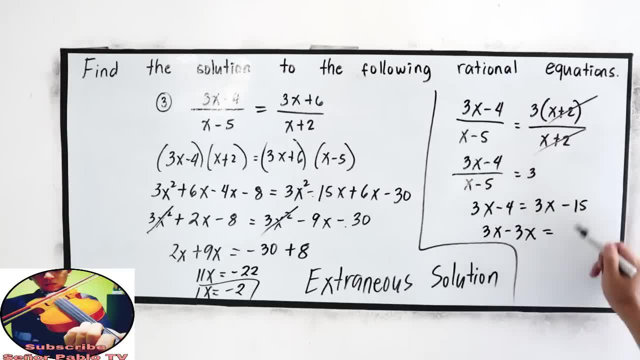 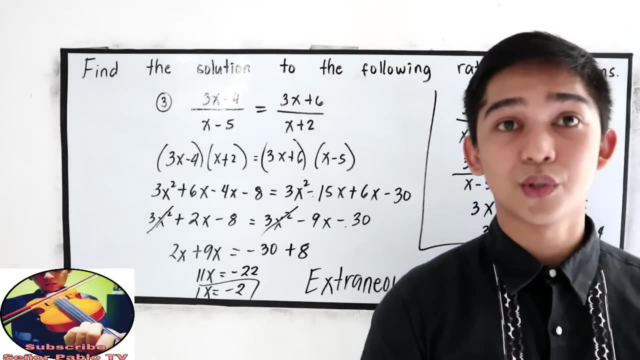 Transpose: 3x-3x is equal to negative 15 plus 4.. This will be cancelled out. 0 is equal to negative 15.. That gives us our extraneous solution. So we don't have solution for this. 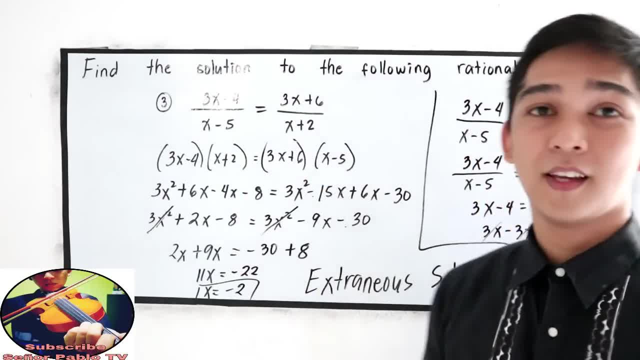 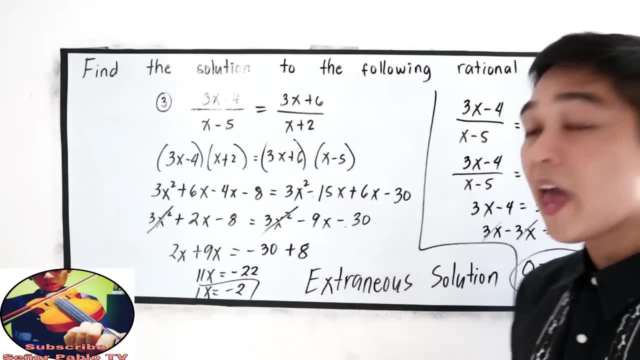 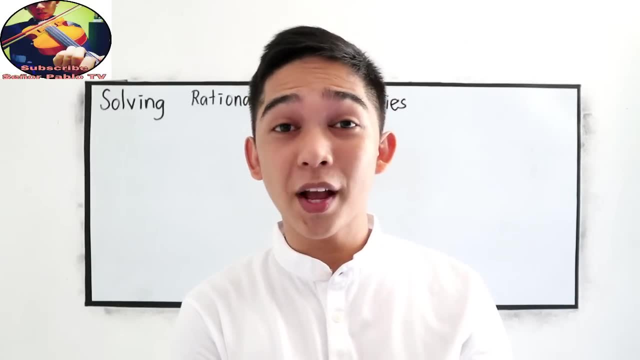 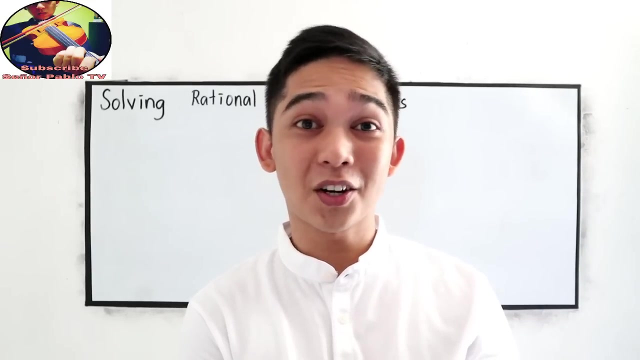 x is empty. So that is our example number 3.. And the introduction form. This is our extraneous solution. Thank you for watching this video. Please make sure that you watch our tutorial video in inequalities and interval notation To better understand this tutorial video. 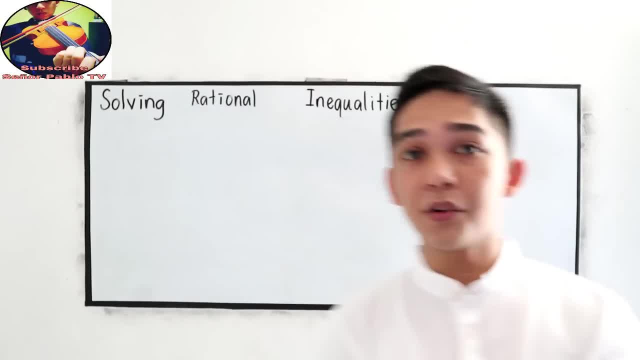 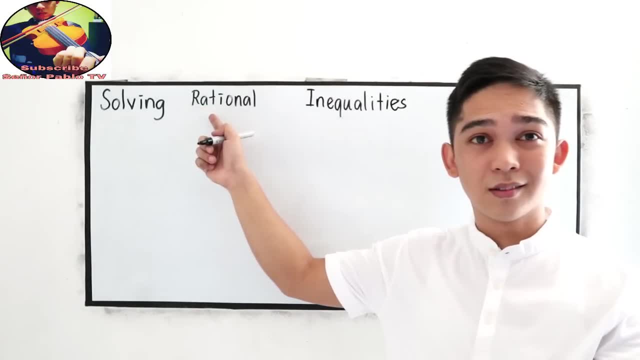 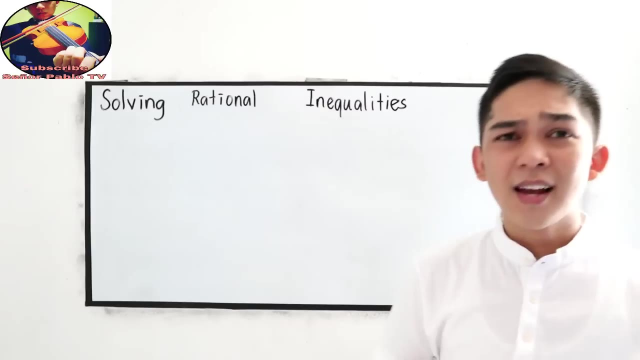 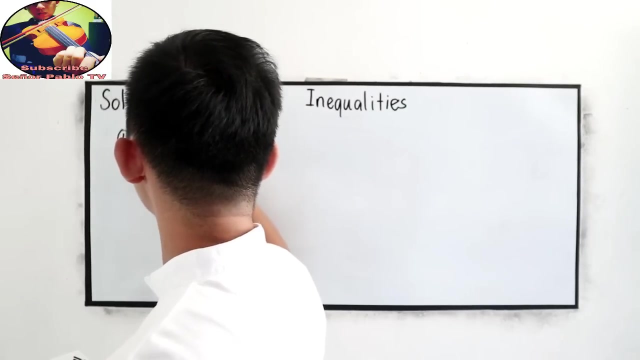 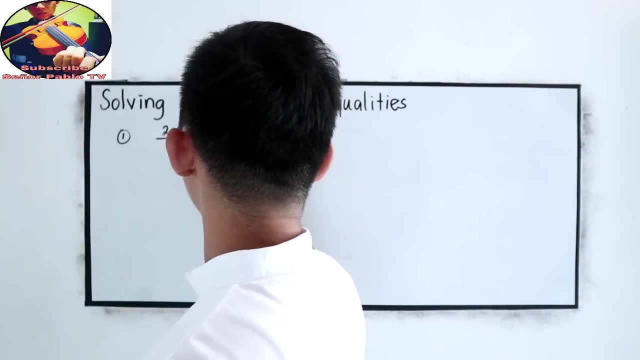 Our topic is solving rational inequalities. Our root word is ratio, So we are dealing with our rational expression, rational inequalities. Let's try number 1.. 2x plus 10 over x plus 3 is greater than or equal to 1.. 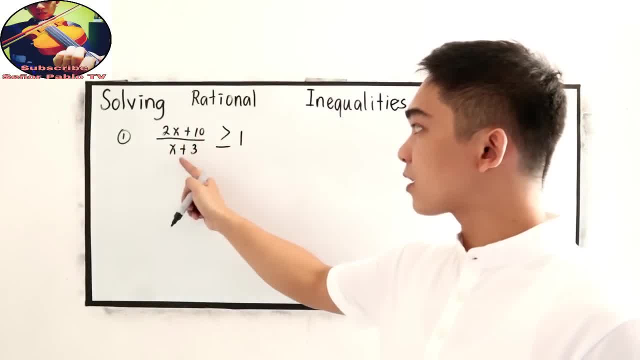 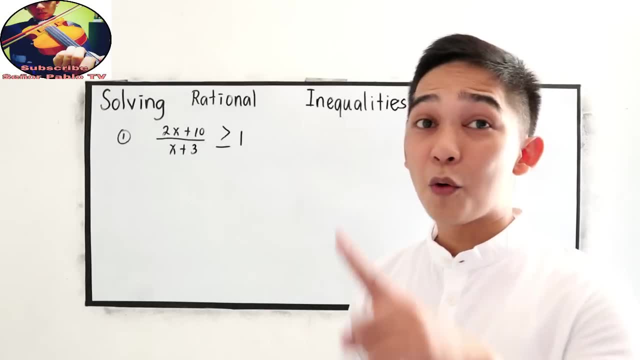 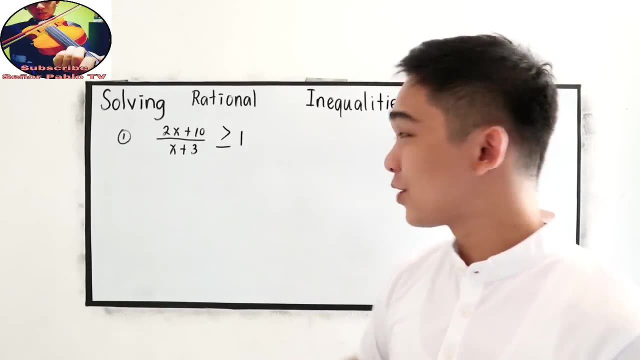 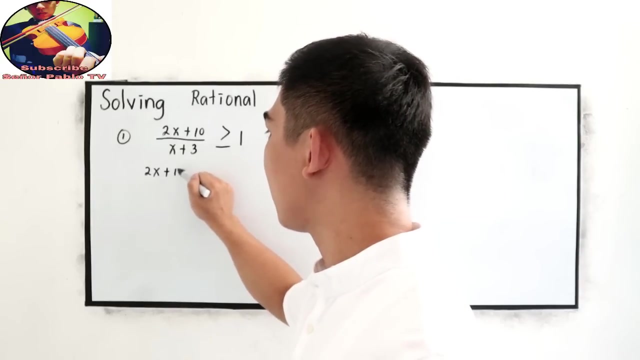 Again, 2x plus 10 over x plus 3 is greater than or equal to 1.. So our first step is our inequality must be equal to 0. So we need to transpose positive 1.. So 2x plus 10 over x plus 3 minus 1.. 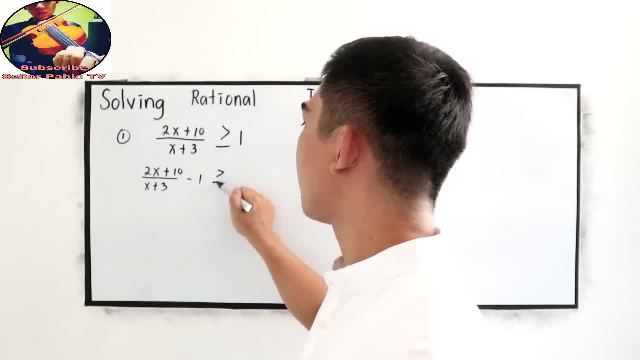 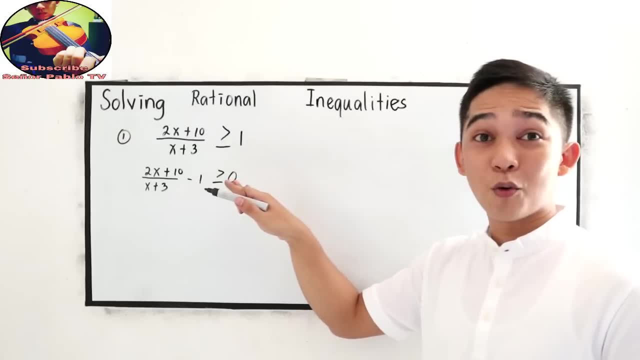 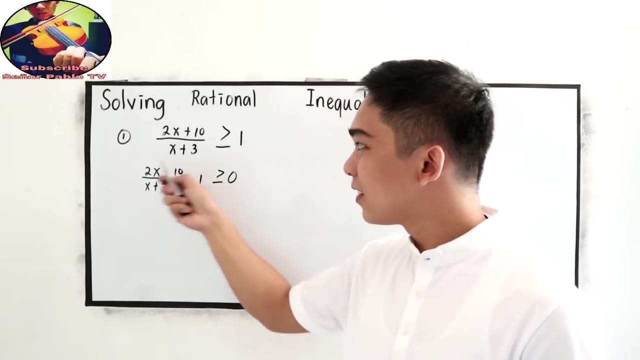 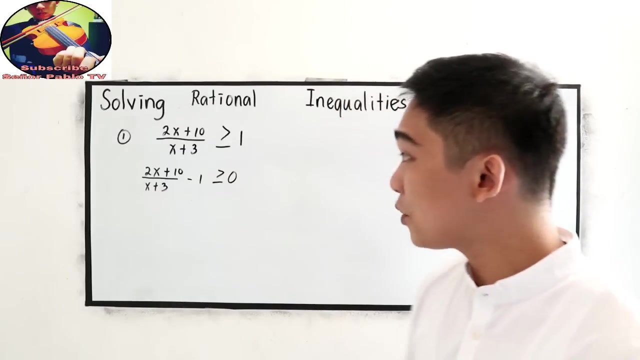 Minus 1 is greater than or equal to 0.. Okay, That is our first step. The inequality must be equal to 0.. Now simplify the left side of our inequality. So we need to find the LCD. Our LCD is: 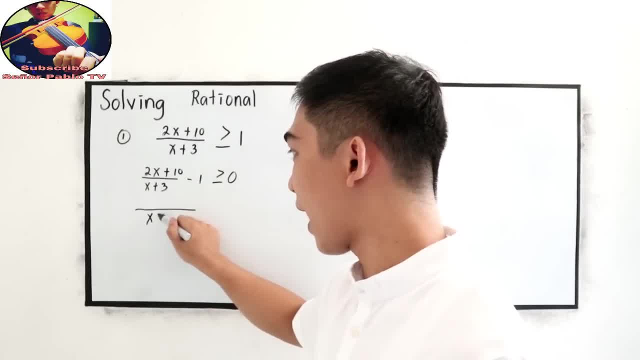 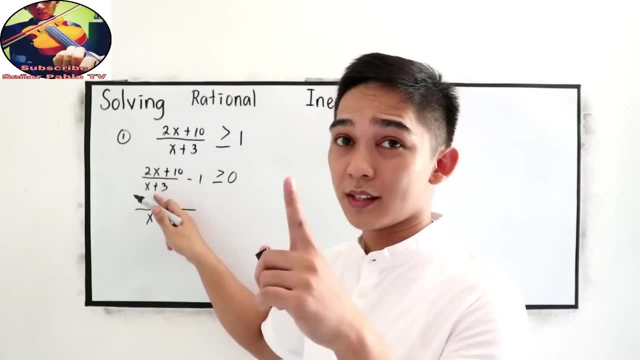 x plus 3. So just copy x plus 3.. x plus 3 divided by x plus 3. That is 1. So 1 times 2x plus 10. So 2x plus 10.. 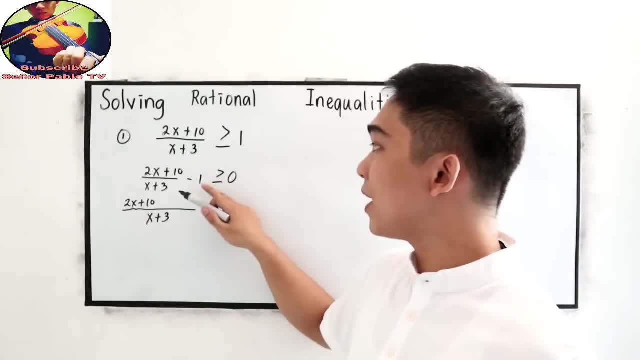 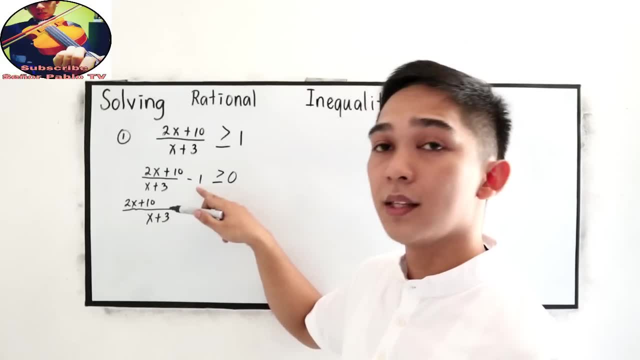 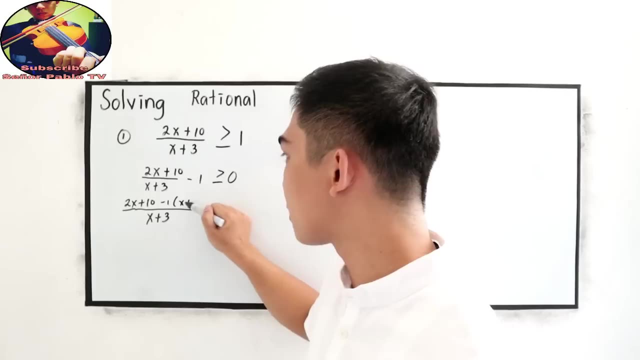 Next, We know that the denominator of 1 is 1.. So x plus 3 divided by 1. That is x plus 3.. Times negative 1. That is negative 1 times x plus 3. Is greater than or equal to 0.. 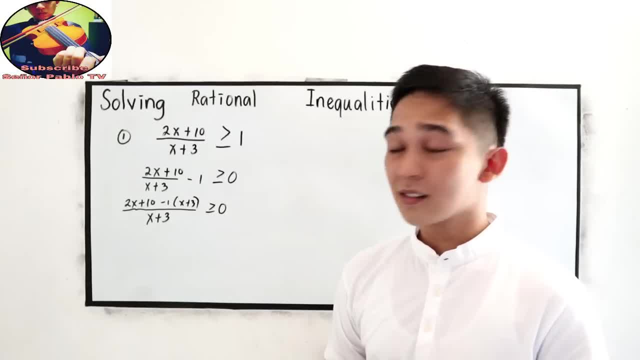 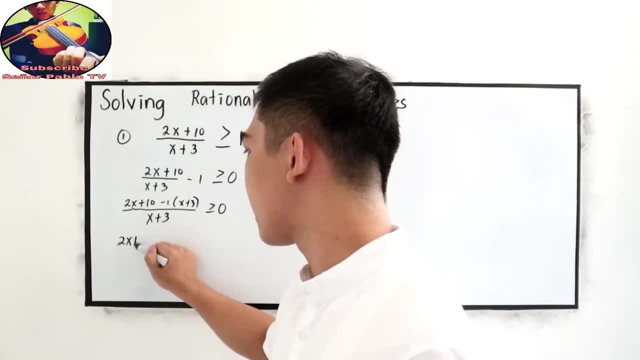 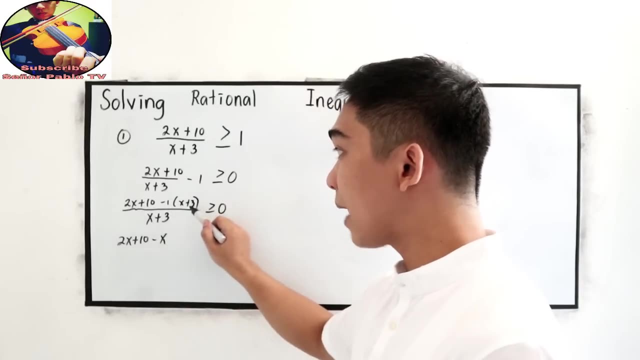 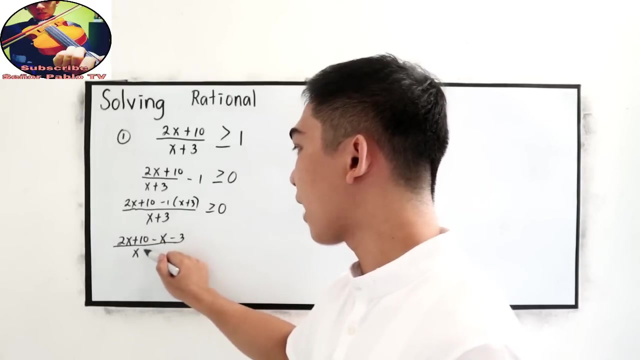 Okay, In this case we need to simplify our numerator, So copy 2x plus 10.. Negative 1 times x. This is negative. x Negative 1 times positive: 3. Negative 3. Over X plus 3.. 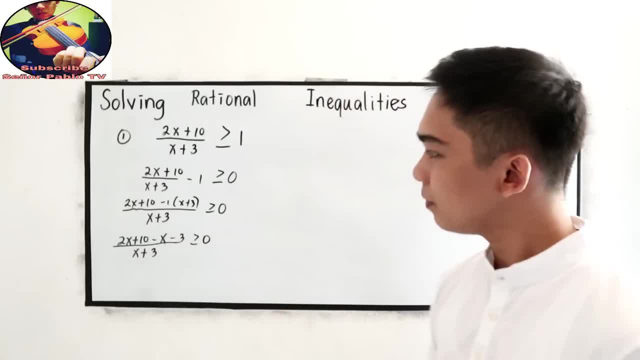 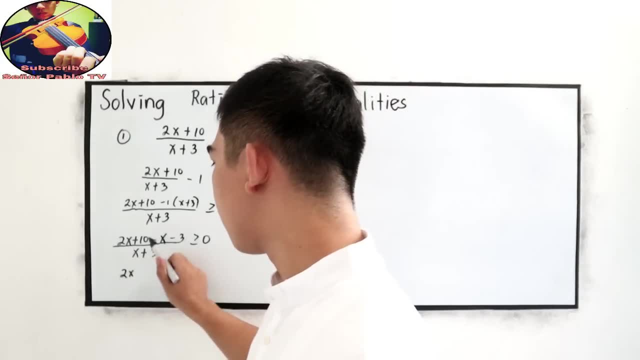 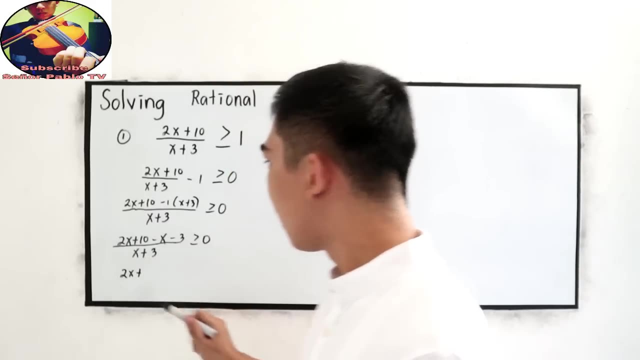 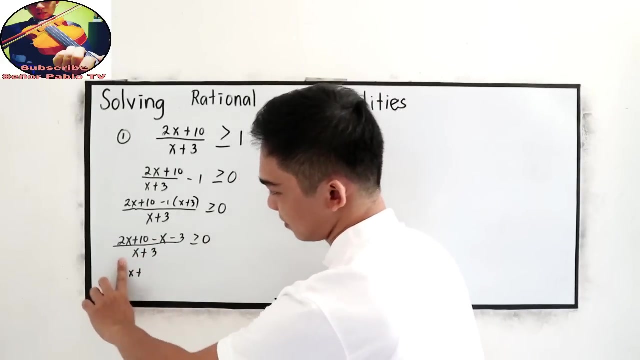 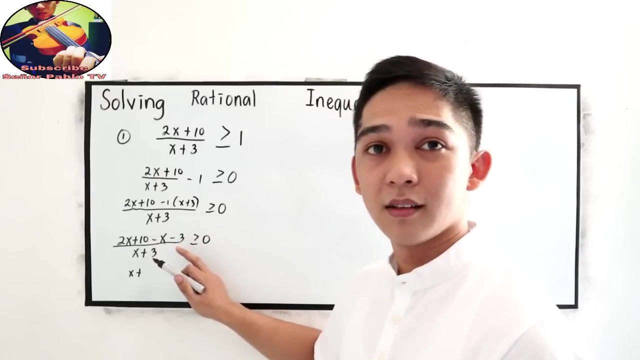 Is greater than or equal to 0. Simplify our numerator. This will become 2x 10 minus 3.. Plus, Okay, We need to combine 2x minus x. that will become x. 2x minus x is x. Next, 10 minus 3, that is positive 7, over x plus 3.. 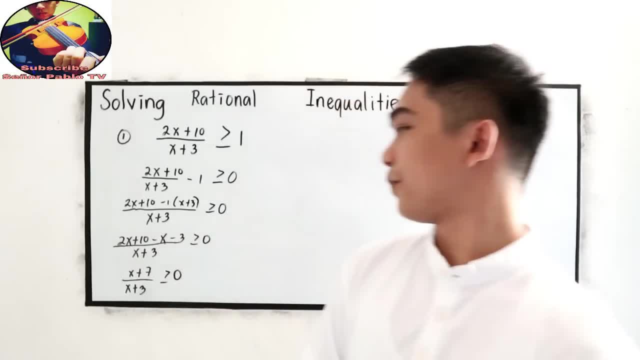 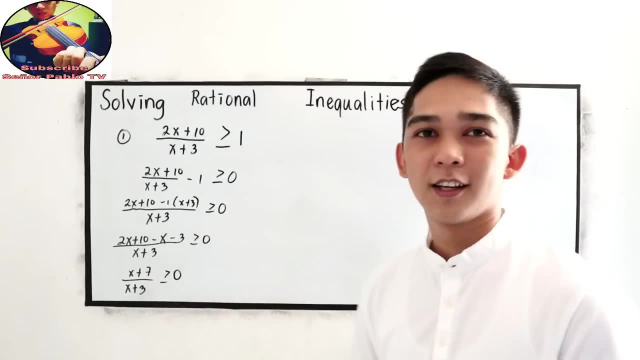 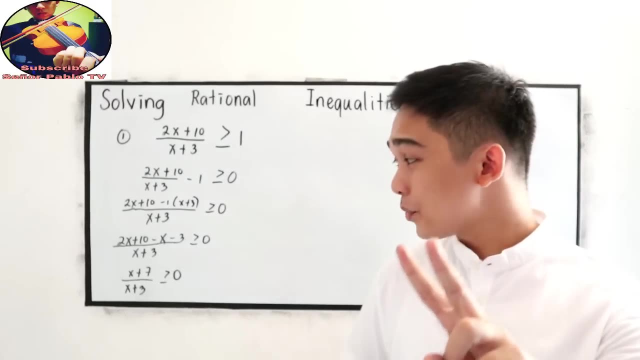 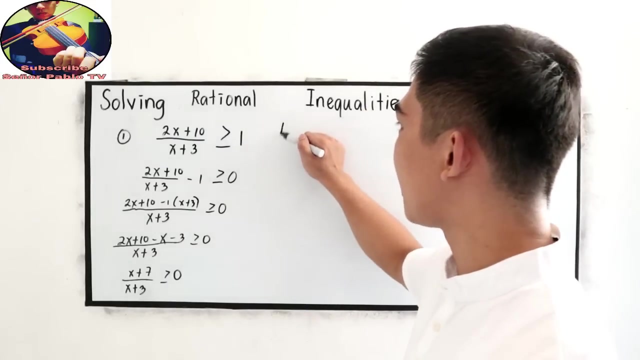 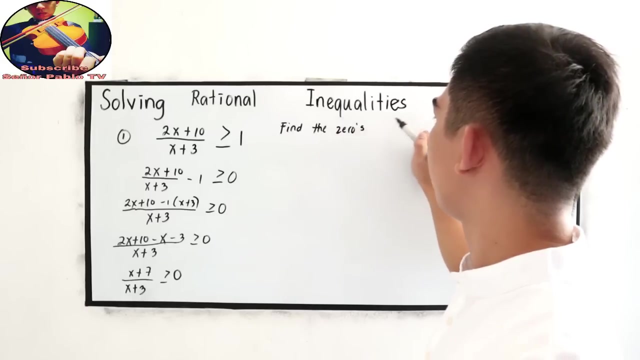 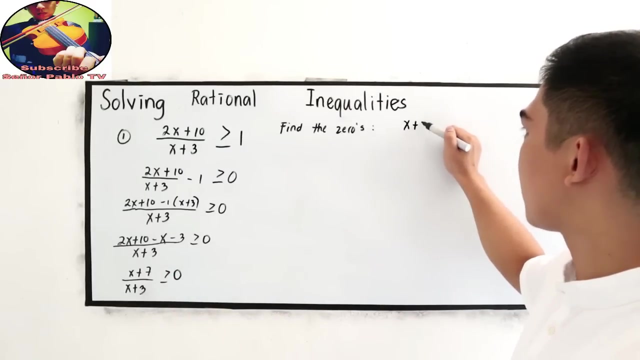 It's greater than or equal to 0.. Okay, That is our simplest form. Now, second step: find the zeros of our rational inequalities. So find the zeros, Zeros. So our zeros are x plus 7, just equate. 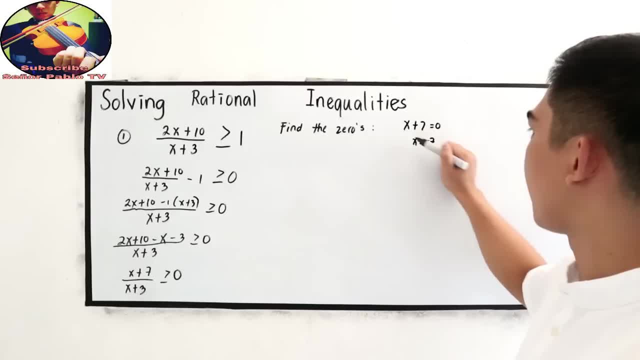 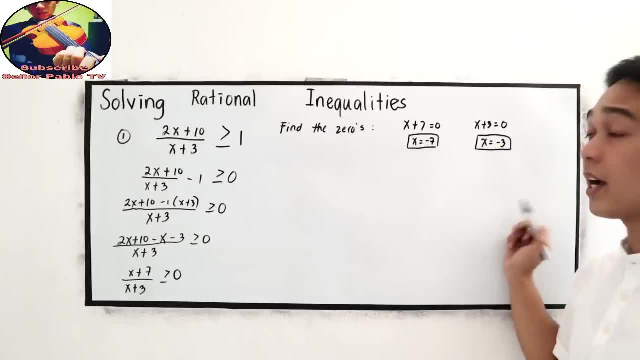 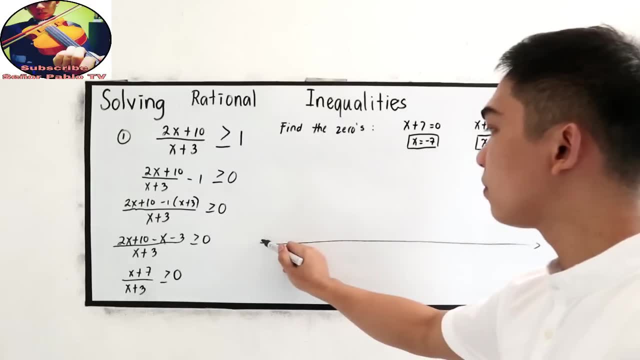 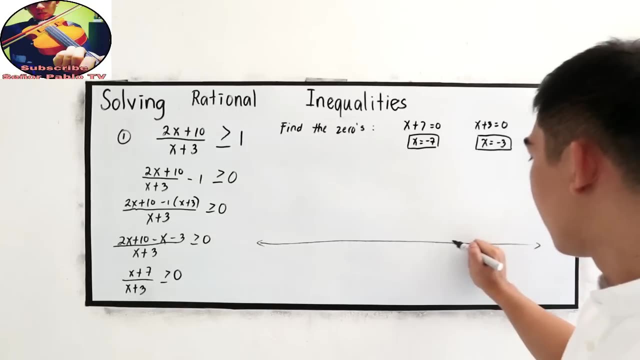 This is now our zeros: negative 7 and negative 3.. Now we need to locate in our number line plot. in our number line Let's say this is our zero: positive 1, positive 2, positive 3.. 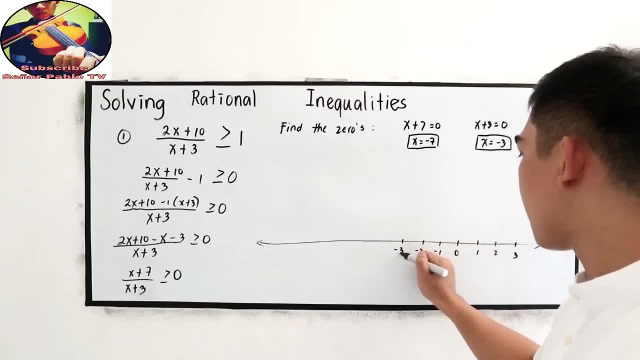 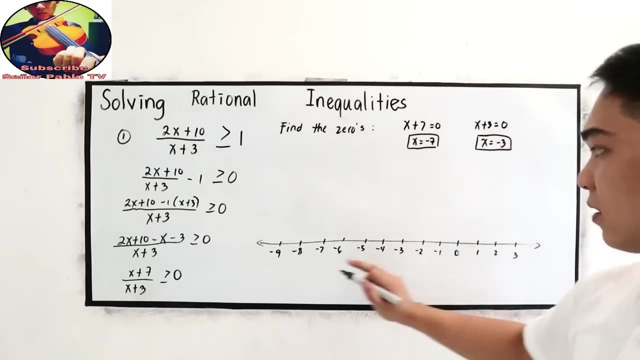 Negative 1, negative 2, negative 3, negative 4, negative 5, negative 6, negative 7, negative 8, negative 9.. Locate negative 7.. Negative 7 is here, Okay, and negative 3.. Now let us check which of the following satisfies our 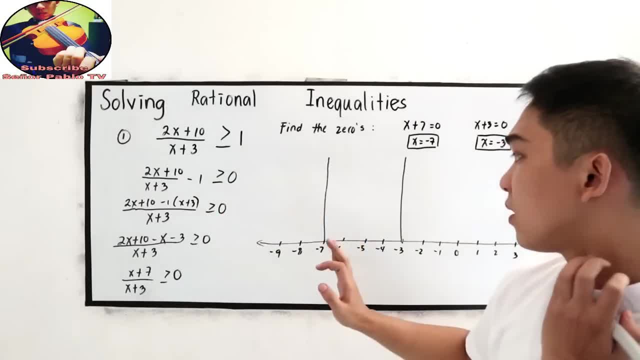 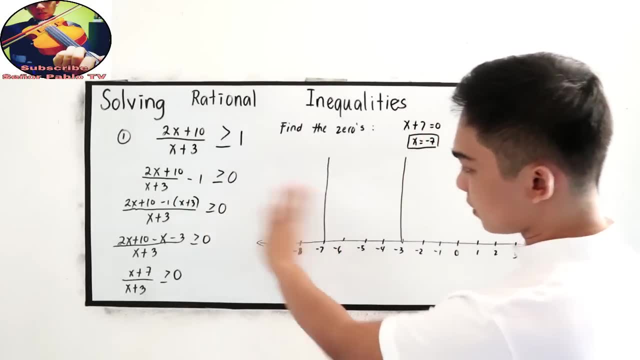 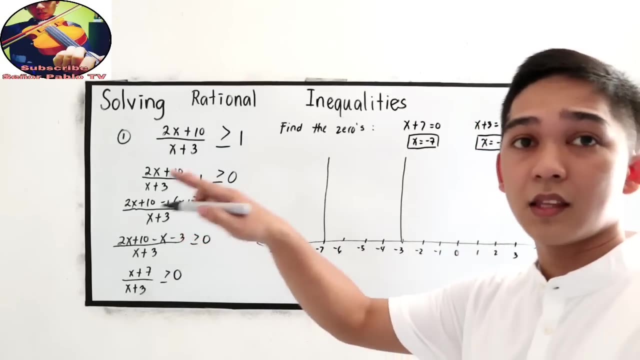 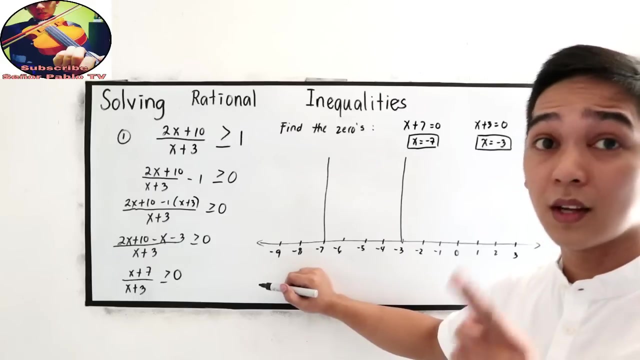 rational inequality. So let us test the leftmost part of our number line. So you need to choose negative 8, negative 9, negative 10, negative 11.. It's up to you. In this case, let us try negative 10.. Will I have negative 10 or negative 9?? okay, let's. 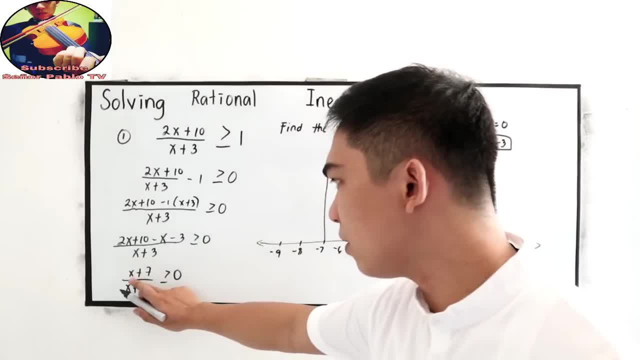 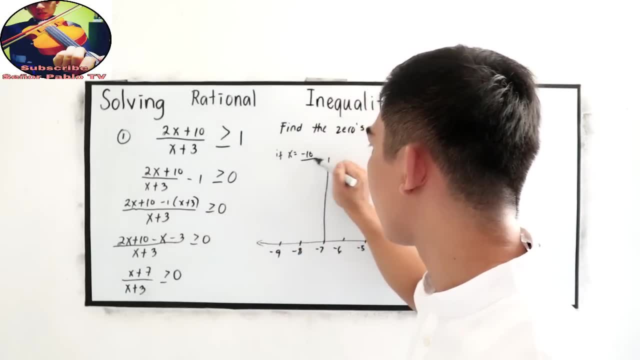 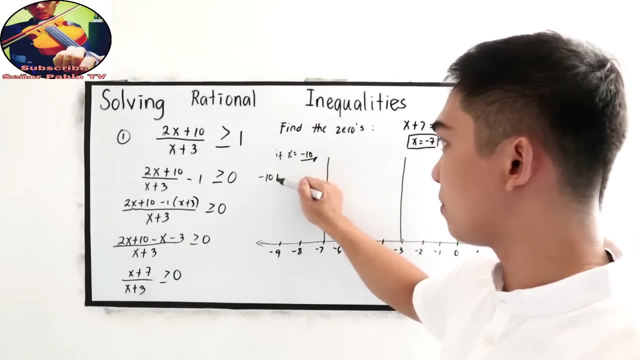 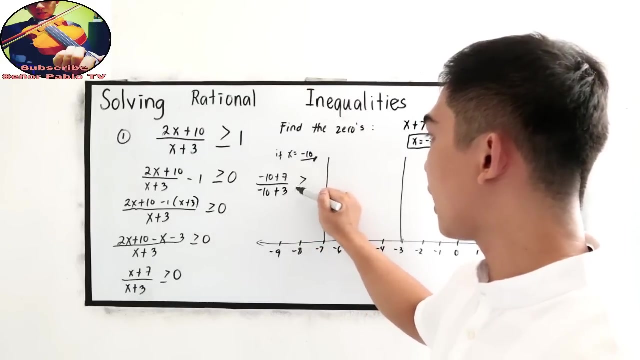 let's choose negative 10.. So substitute our value of x to negative 10.. If x is equal to negative 10.. so So negative 10, just change to negative 10. or substitute plus 7 over x is negative 10 plus 3, greater than or equal to 0.. 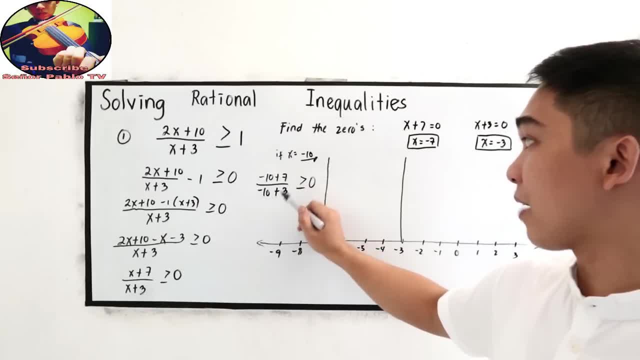 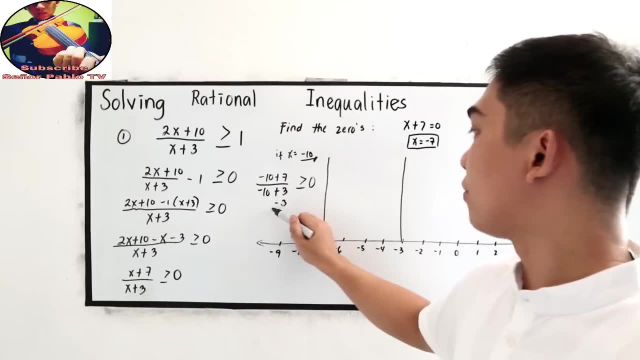 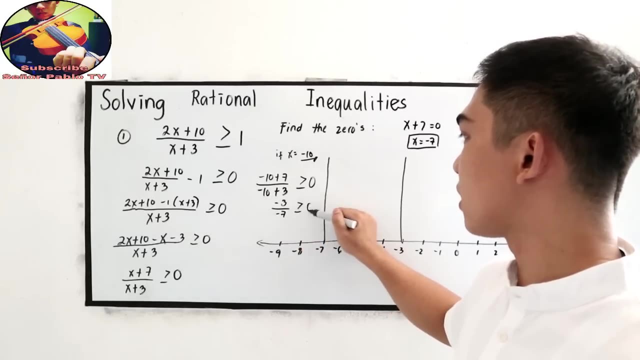 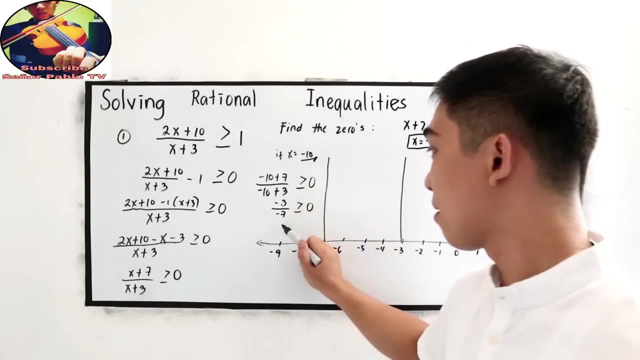 So negative 10 plus 7 is negative 3 over negative. 10 plus 3, negative 7, greater than or equal to 0.. Negative divided by negative, that will give us positive 3 over 7, greater than or equal to 0.. 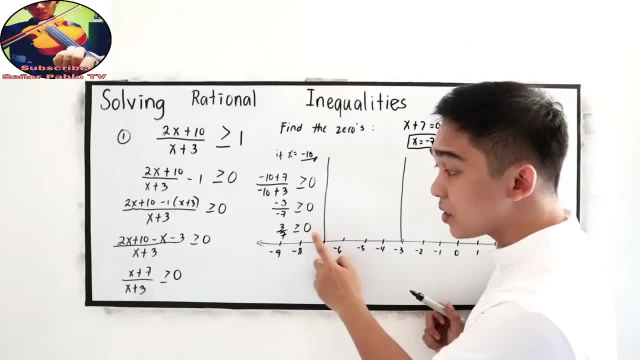 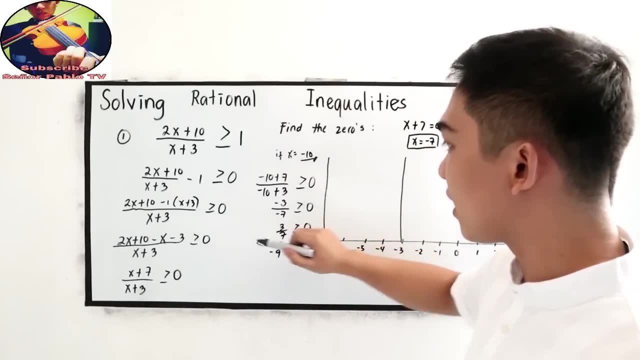 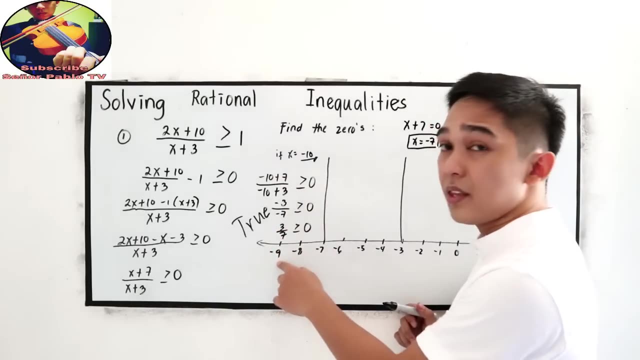 3 over 7, is it greater than 0?? Yes, it is So. if x is negative 10,, this is true. Okay, Of course, if x is negative 9, that is also true. And if x is negative 8, that is also true. 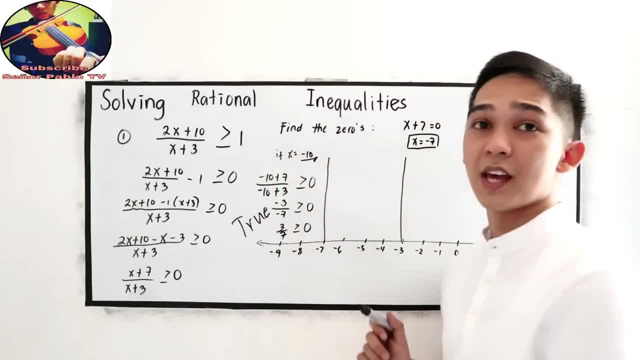 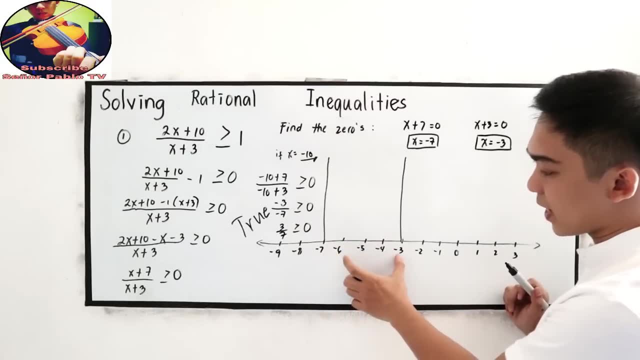 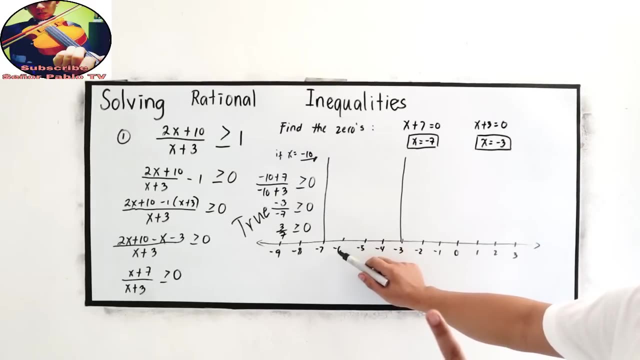 All the numbers on the left side, all negative 7.. Now let us test the numbers. Let us test the numbers between negative 7 and negative 3.. So pick one number: either negative 6,, negative 5, or negative 4.. 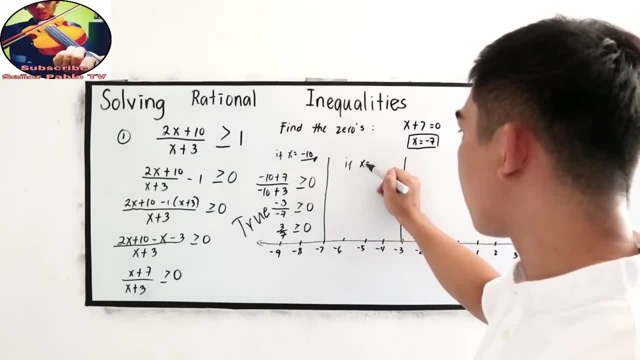 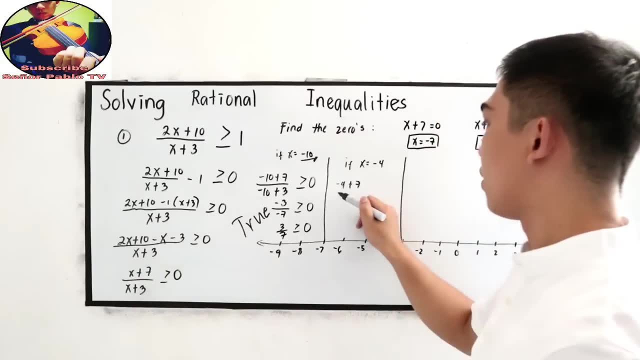 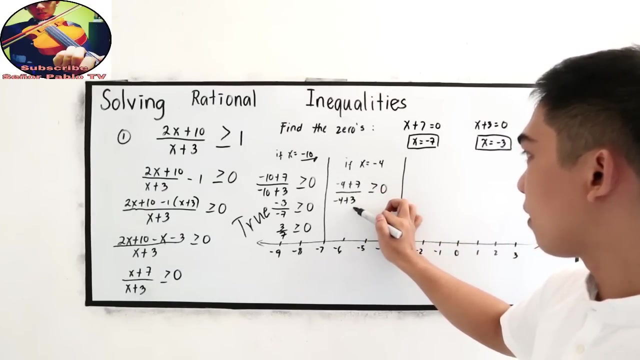 Let us choose negative 4.. If x is equal to negative 4, then substitute negative 4 plus 7 over negative 4 plus 3, is it greater than or equal to 0?? Now let us check Negative 4 plus 3,, that is positive 3, over negative 4 plus 3, negative 1, greater than or equal to 0. 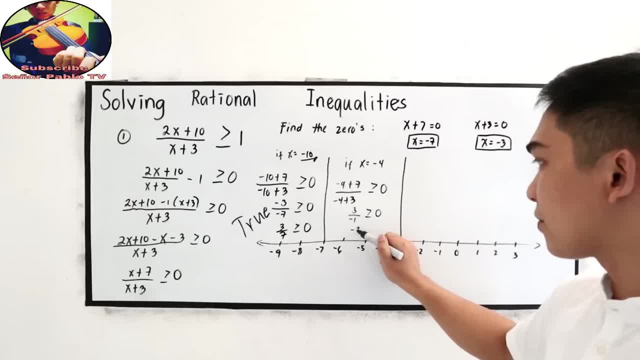 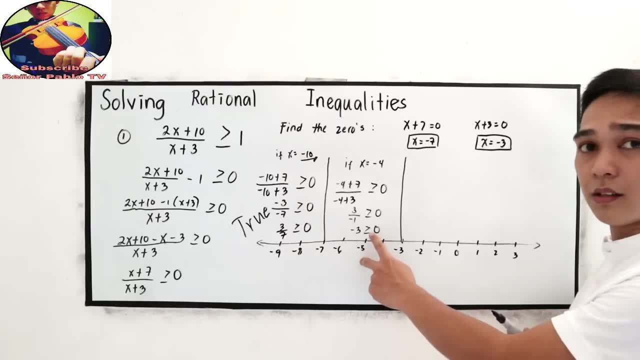 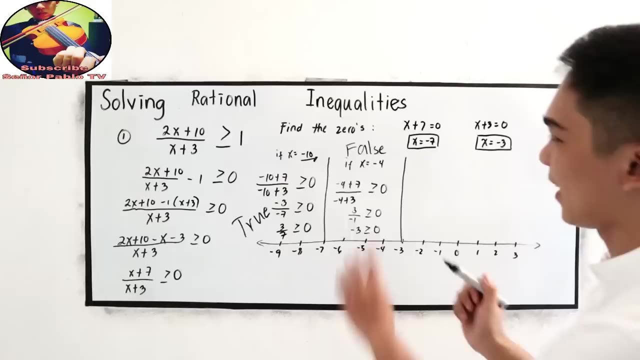 3 divided by negative 1, that is negative 3, greater than or equal to 0.. Is negative 3 greater than 0?? No, So this is false. Okay, So the following numbers are not included: negative 6,, negative 5, and negative 4.. 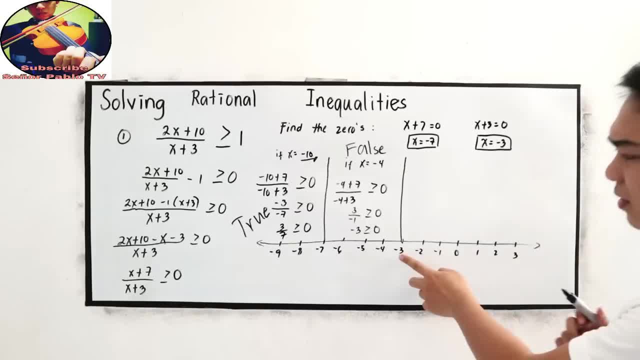 How about the numbers on the right side of negative 3?? So let us check 0, because 0 is the easiest one. So if x is equal to 0, so 0 plus 7 over 0 plus 3, greater than or equal to 0. 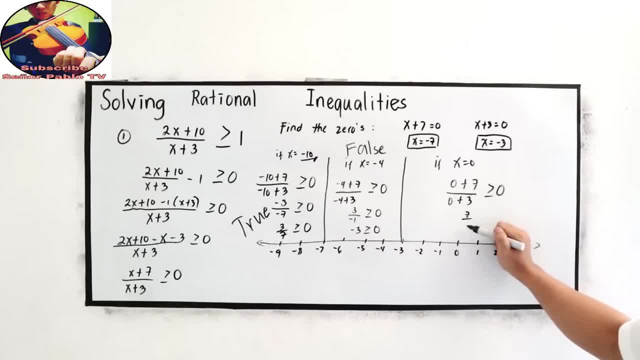 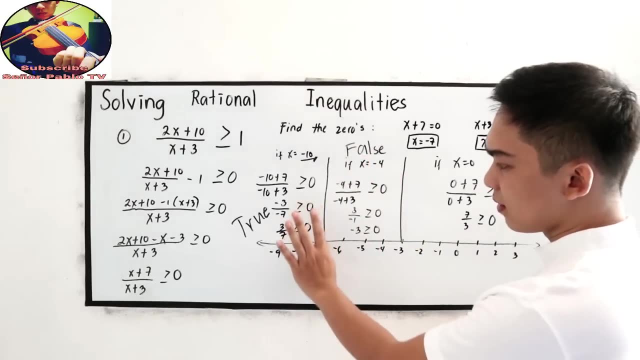 0 plus 7,, 7 over 0 plus 3, 3, greater than or equal to 0.. 7 over 3 is greater than 0?? Yes, So this is true. So we are going to get the left side. 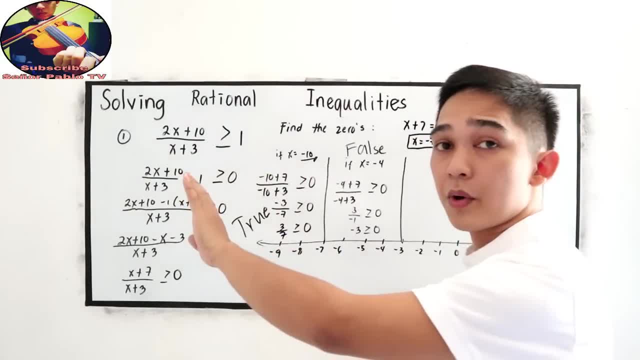 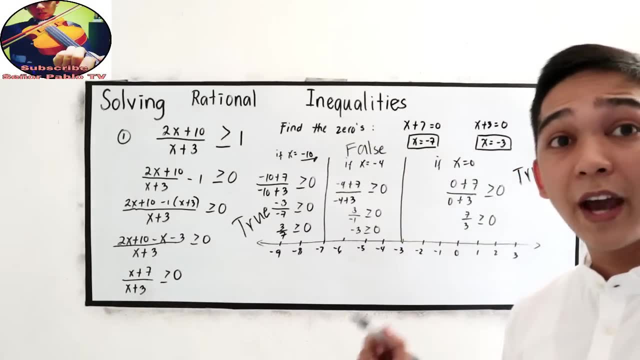 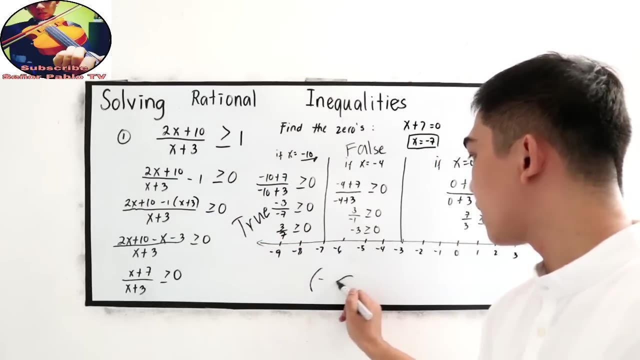 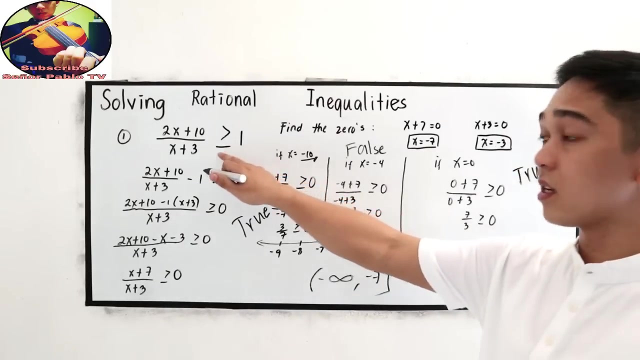 of negative 7, because that will make our inequality correct, and the right side of negative 3.. So to write our final answer: open to negative infinity and 7, that is close. Why close? Because that is equal to greater than or equal to union. 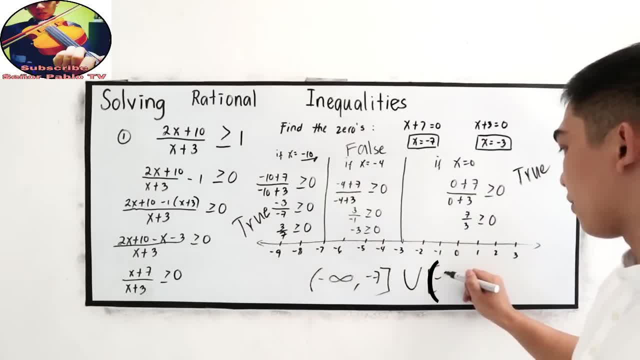 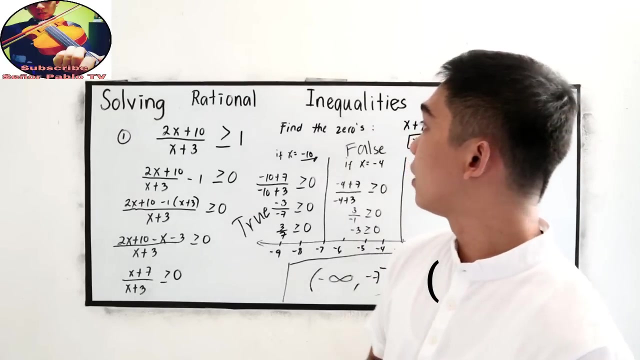 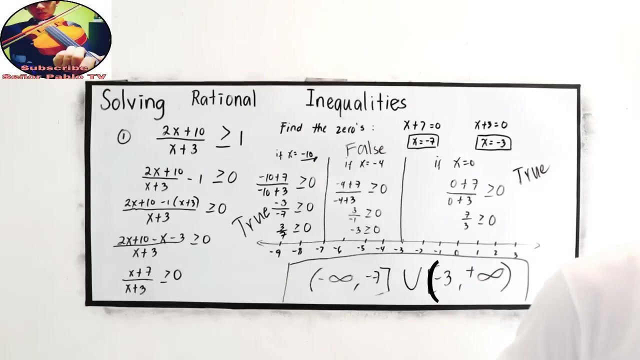 negative 3 going to positive infinity. This is now our final answer: Negative infinity to negative 7, close Union, close to negative 3 to positive infinity. So that is on how to solve rational inequalities. Now let's I want you to solve. 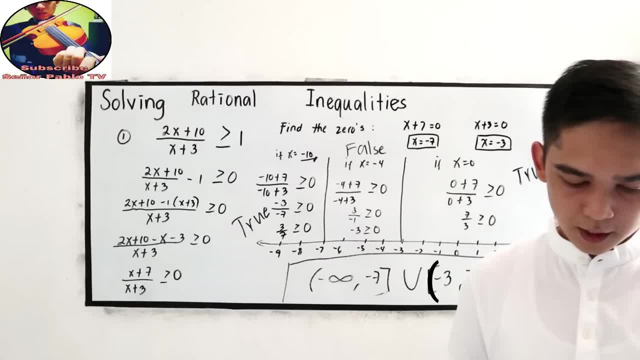 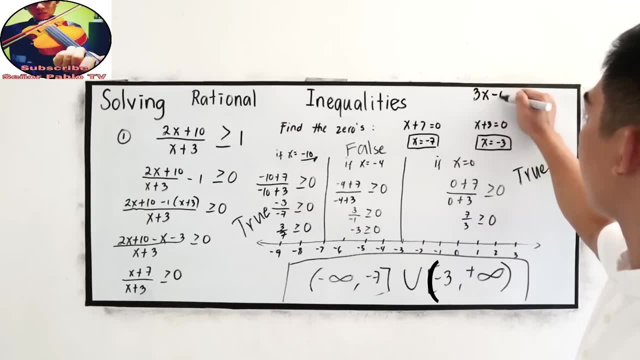 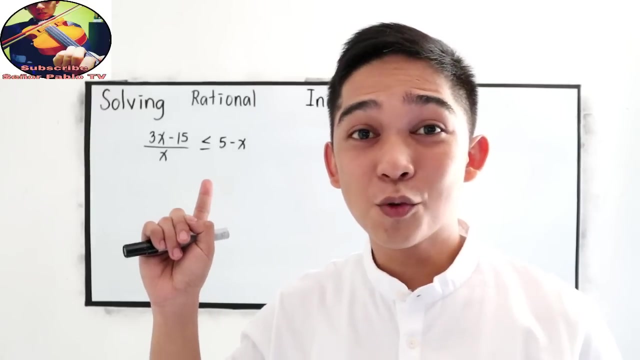 this problem: 3, 3x minus 15 over x, less than or equal to 5 minus x. Try to solve this. 3x minus 15 over x is less than or equal to 5 minus x. This will be the checking of the problem. 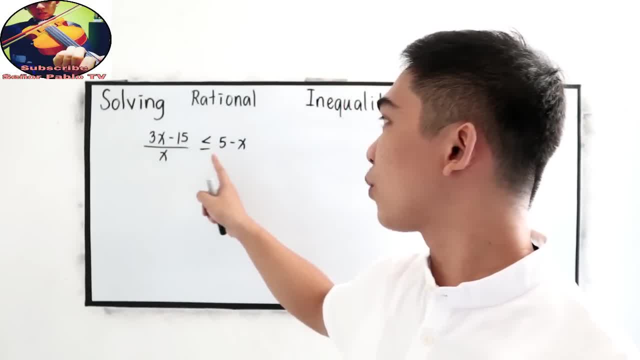 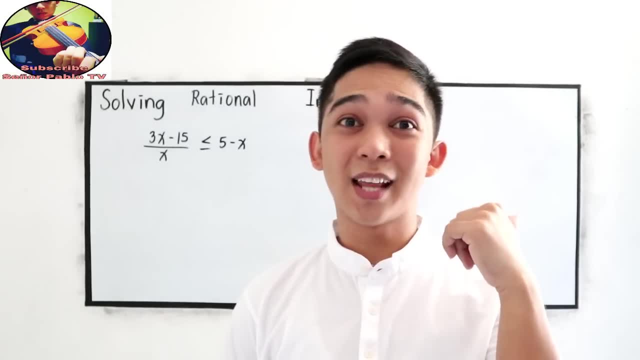 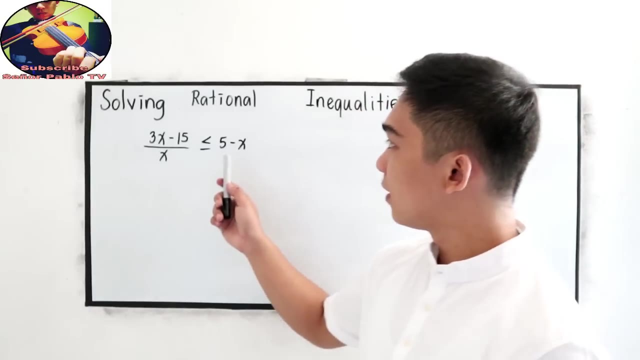 3x minus 15, over, x, less than or equal to 5 minus x. That is your assignment in our tutorial video last time in problem number 1.. Now let us check your work. Our first step is to check your work. Our first step is to check your work. 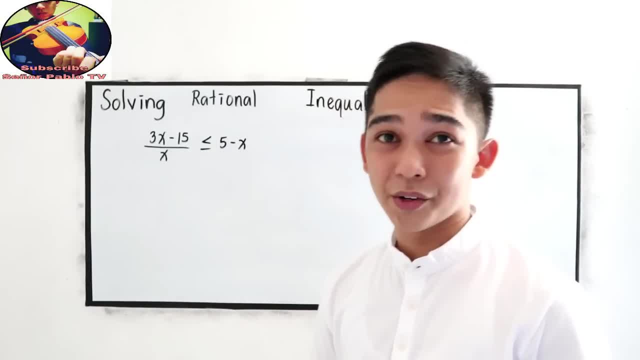 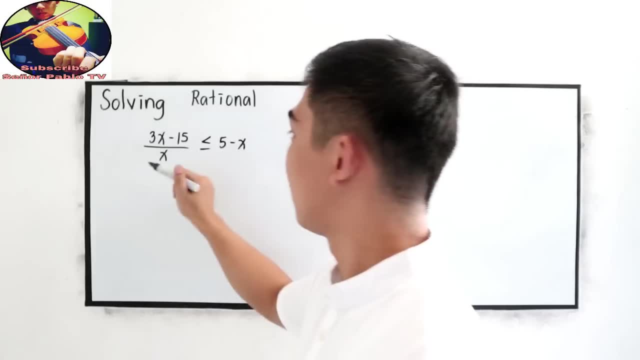 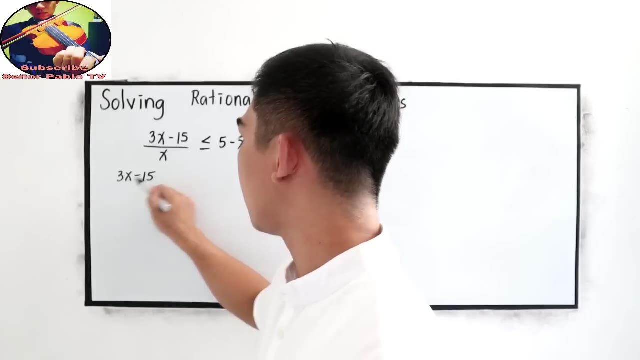 The inequality must be equal to 0.. The inequality must be equal to 0. So let us move 5 minus x on the left side. So use the addition property of equality: 3x minus 15 over x minus 5 plus x. 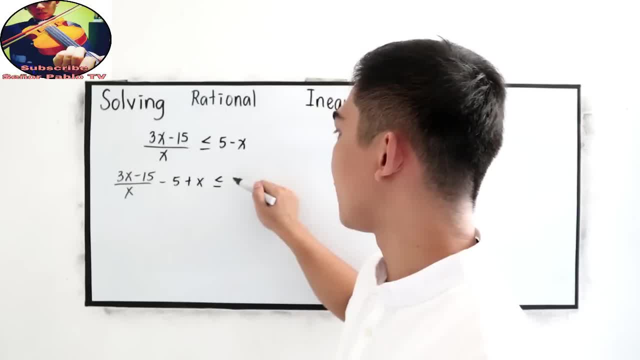 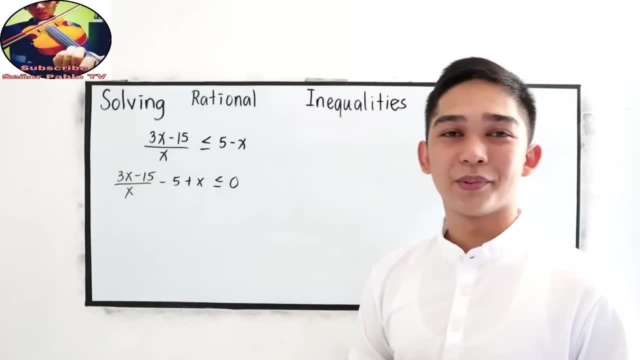 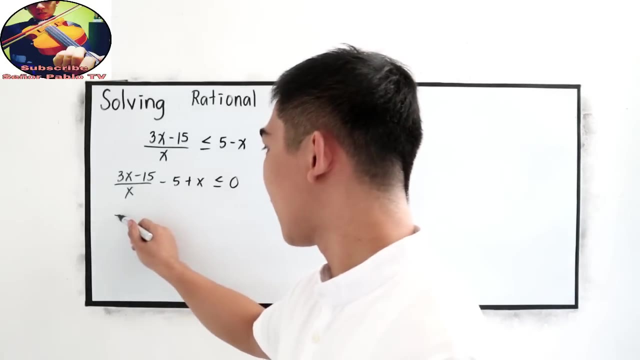 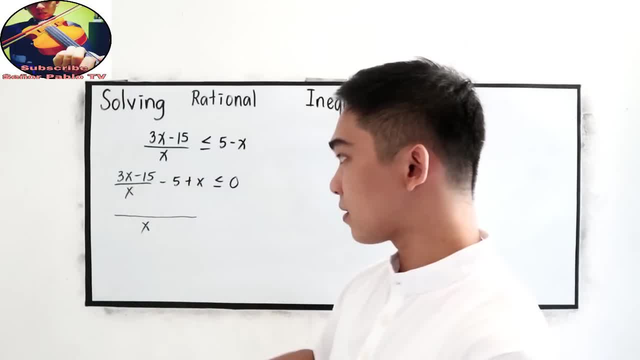 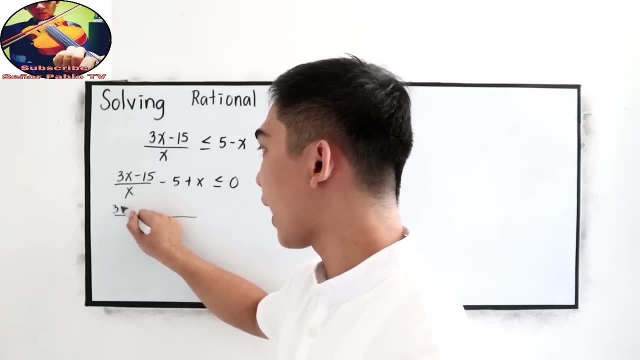 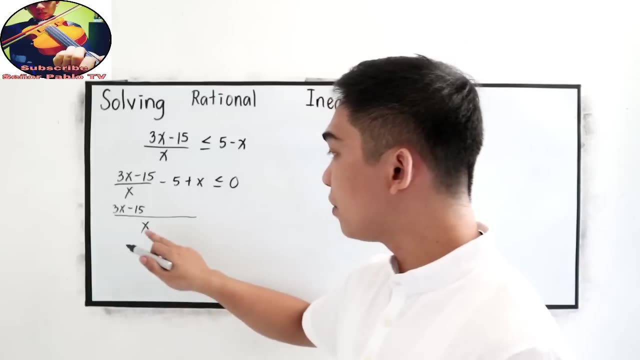 our denominator. So x divided by x, that is 1 times 3x minus 15. that will give us 3x minus 15, or just copy it. this is all already equal to x. now x divided by one. we have a denominator of one here. 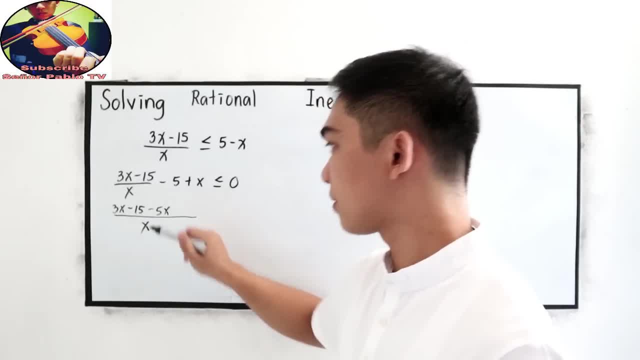 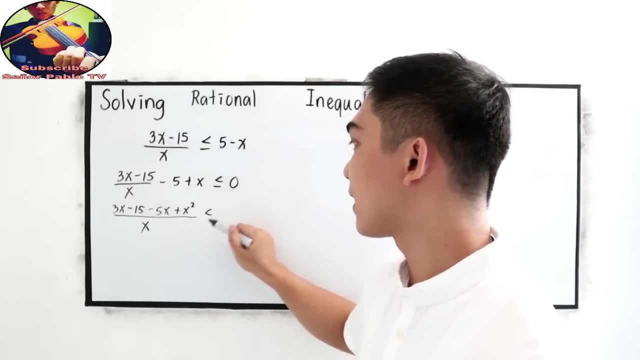 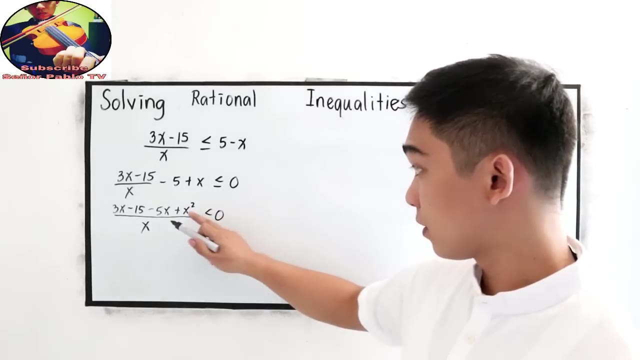 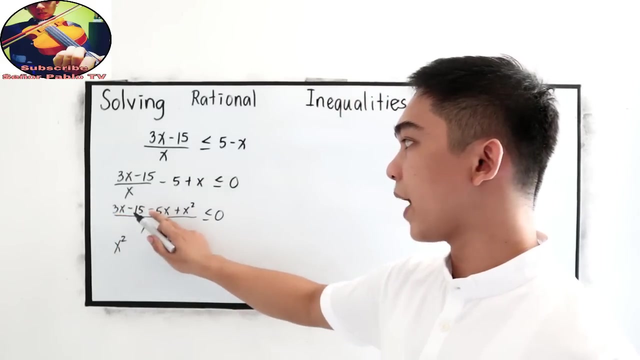 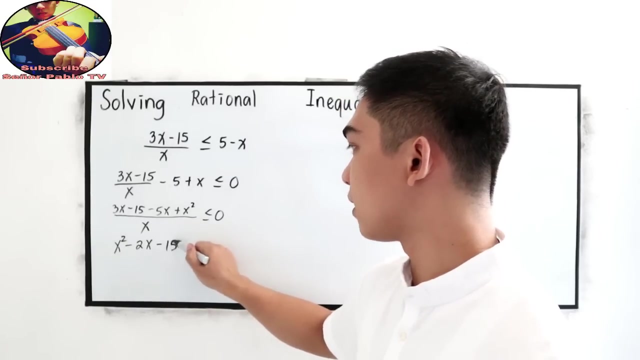 times negative, five negative, five, x and x divided by one times x. positive, x squared, it's less than or equal to zero. now simplify our numerator. then arrange from descending order. so: x squared: three x minus two minus five x. negative, two x minus 15 on over, x is less than. 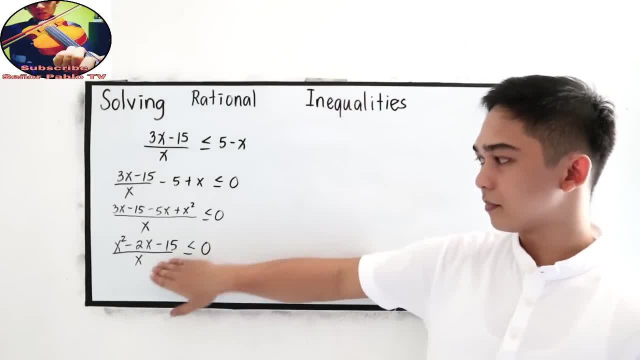 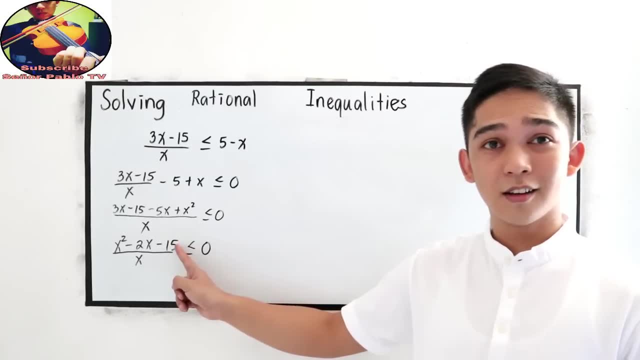 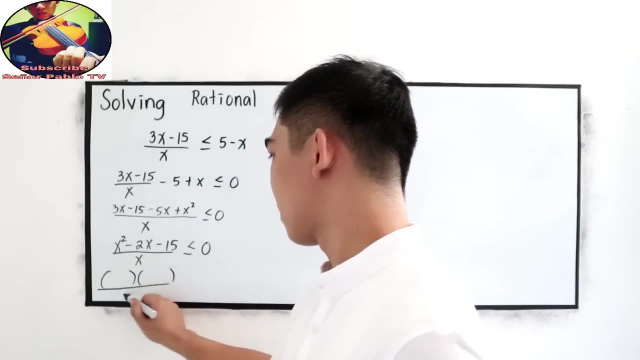 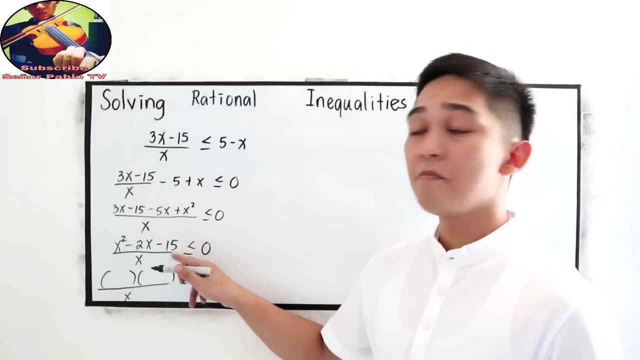 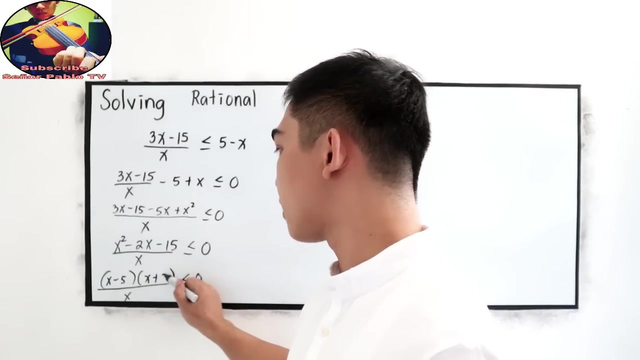 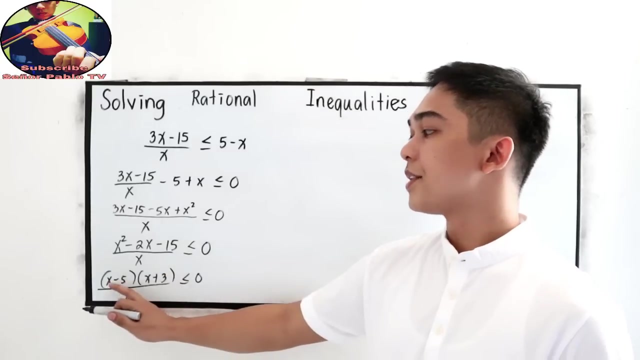 or equal to zero. okay, now, since this is quadratic, find the factors. so factors are factors of negative 15. the sum must be negative 2x, so that is x minus 5 and x plus 3. let's check: negative 5 times positive, 3, negative 15.. negative 15 times 3, negative, 2.. okay, 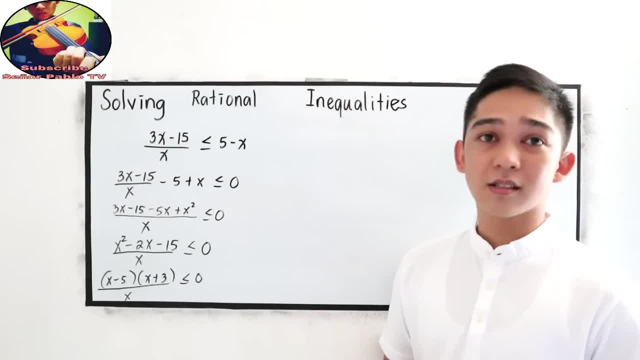 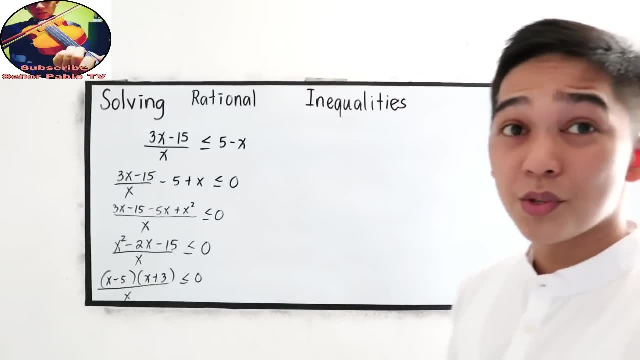 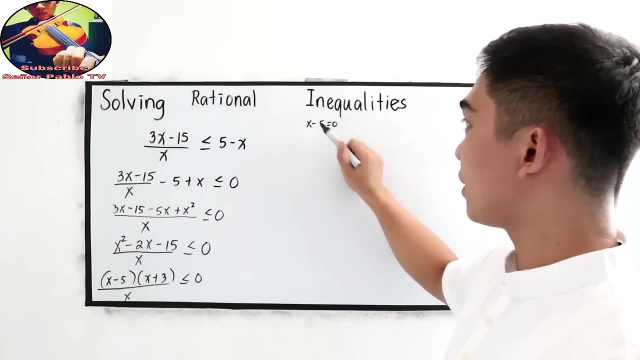 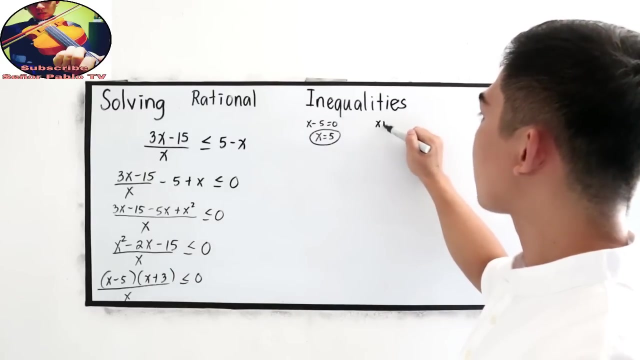 so for our next step, find the zeros of our inequality. so just equate to zero: x minus 5 is equal to zero, that will become x is equal to five, so the zeros are five. the other one, x plus three, is equal to zero, so x is negative three. 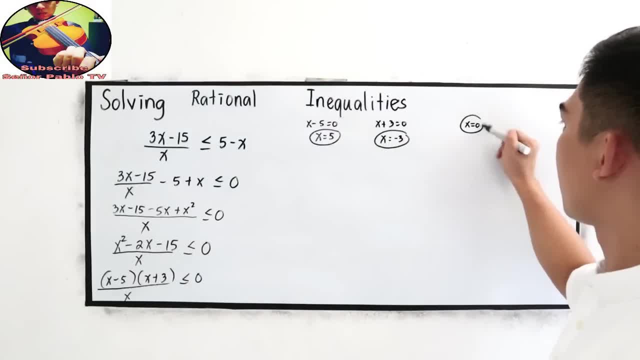 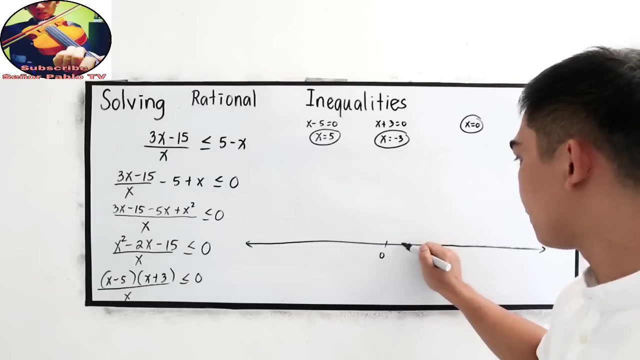 or for the denominator x is equal to zero. so the zeros are five negative three and zero. now our number line. so let's say zero one, two, three, four, five. i will adjust it on the middle part. let's say zero one, two, three, four, five, six, seven. negative one, negative two, negative three. 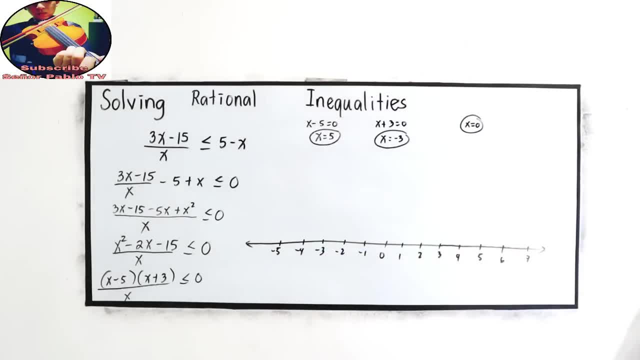 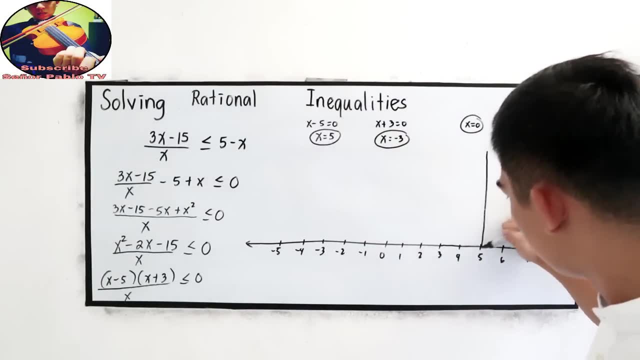 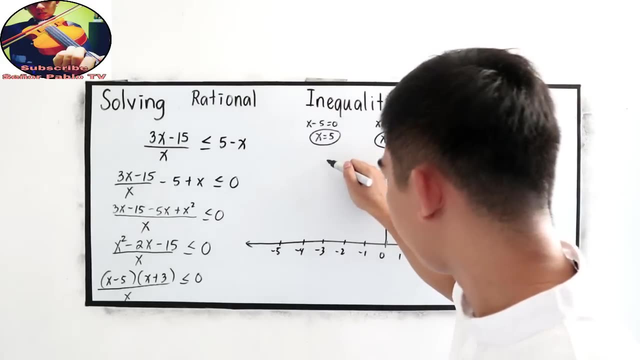 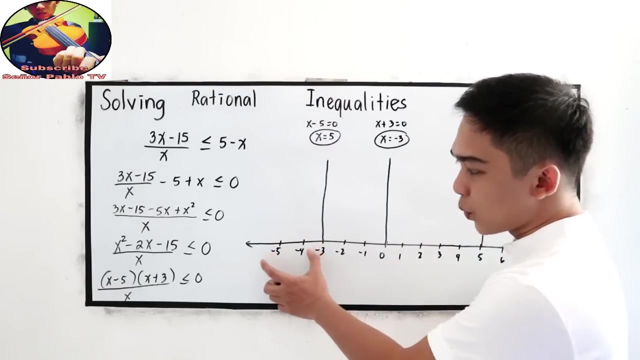 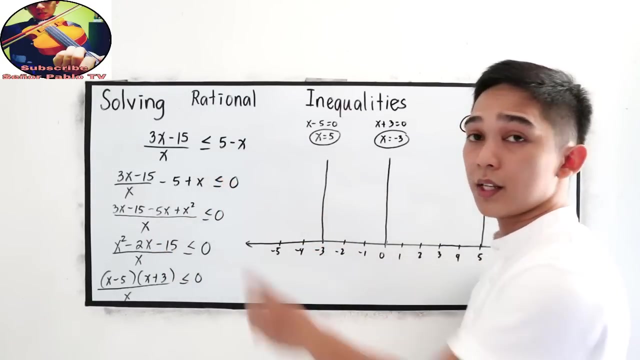 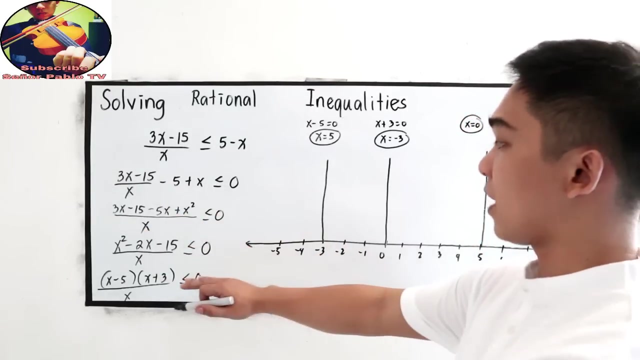 negative four and negative five. now locate our zeros pasting five. here you have the zero and negative three. okay, that's it. let us test whether the numbers on the left side of negative three satisfies our inequalities. choose between negative five, negative six, negative four or not negative seven. 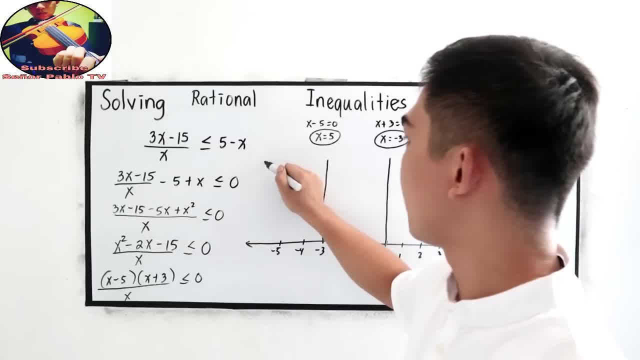 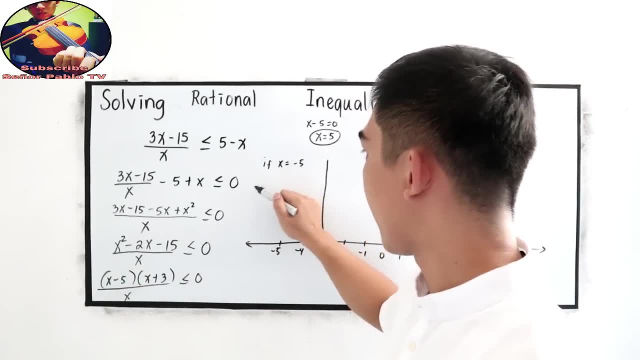 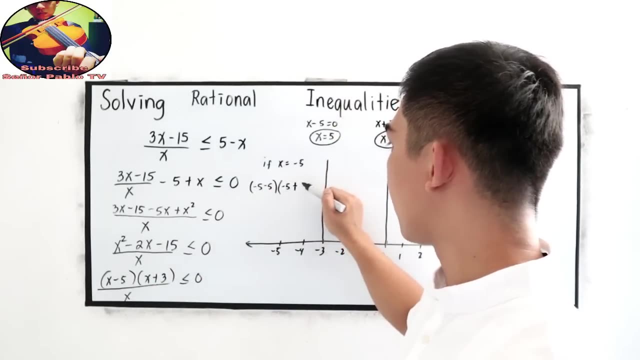 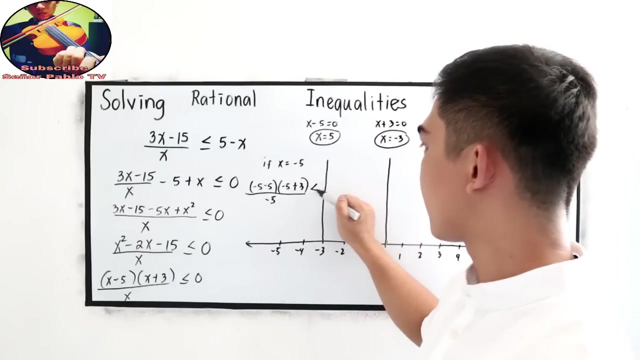 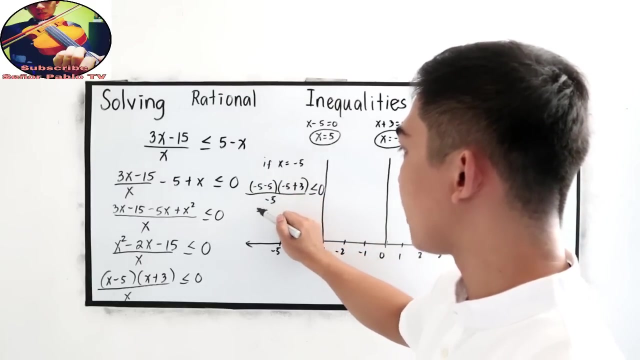 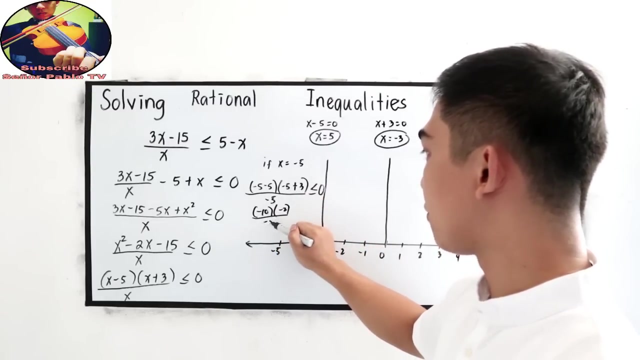 okay, let's try five. so if x is equal to negative five, so negative five minus five. negative five plus three over negative five is less than or equal to zero. Let's check Negative 5 minus 5, this is negative 10.. Negative 5 plus 3, negative 2, all over negative 5.. Negative 10 times negative 2, that is 20 over negative 5.. 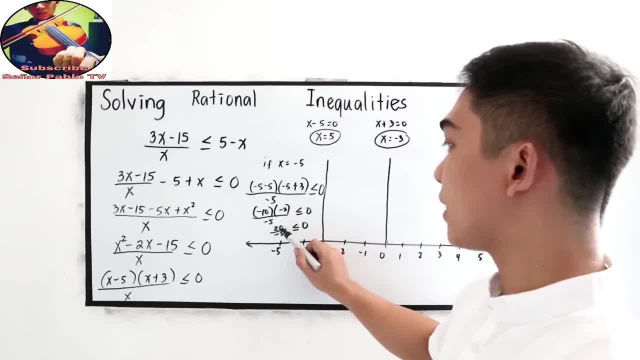 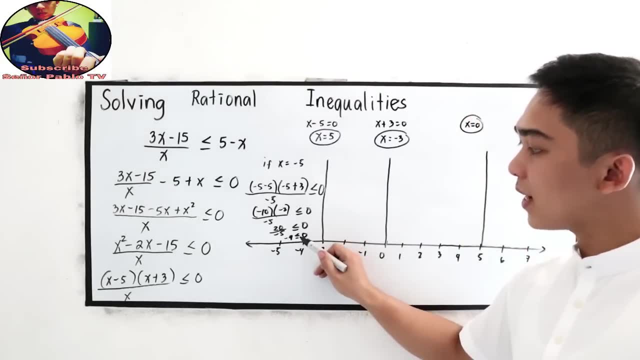 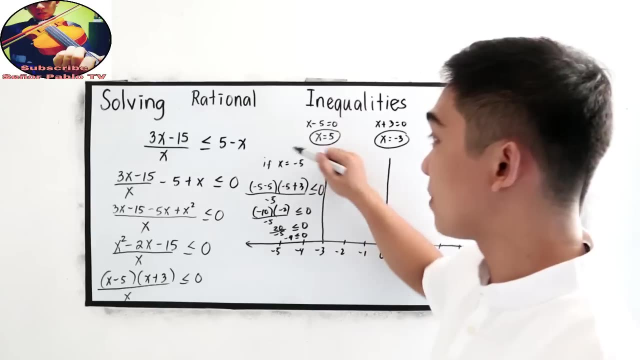 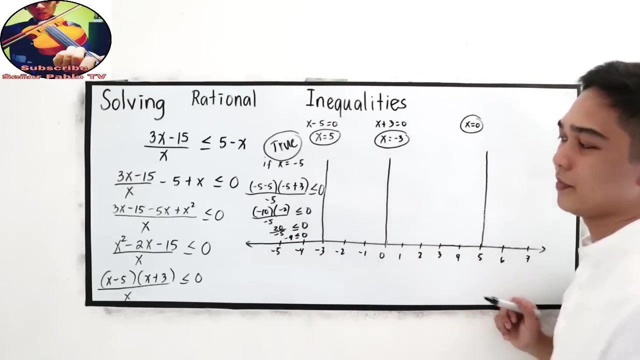 20 divided by negative 5, negative 4 is less than or equal to 0.. Is negative 4 less than or equal to 0?? Yes, so that means this is true. Negative 4 is less than 0.. Now let us check this. 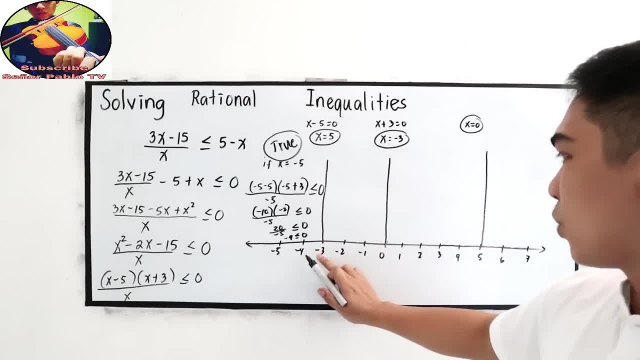 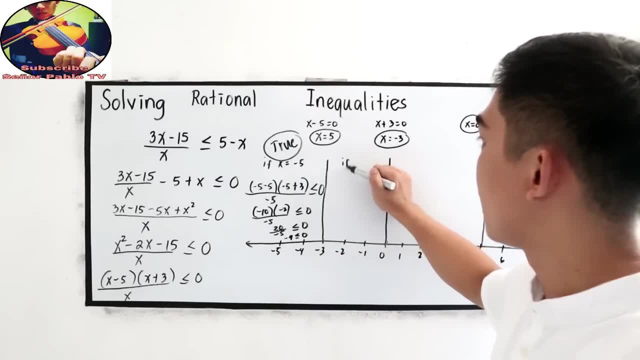 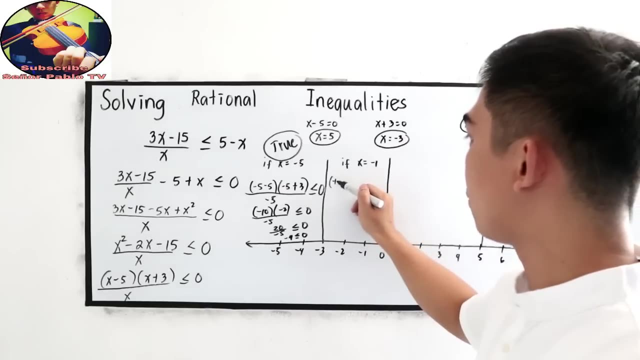 This is numbers between negative 3 and 0.. Choose between negative 2 and negative 1.. Let us try negative 1.. If x is equal to negative 1. So we have negative 1 minus 5, negative 1 plus 3 over negative 1 less than or equal to 0.. 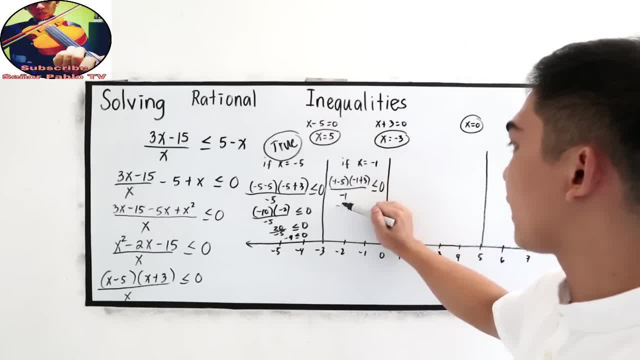 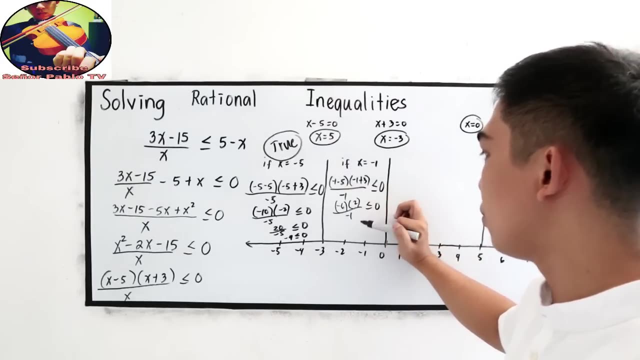 Negative 1 minus 5.. That is negative 6 times negative. 1 plus 3,. 2 over negative 1 less than or equal to 0.. Negative 6 times 2, that is negative 12 over negative 1 less than or equal to 0.. 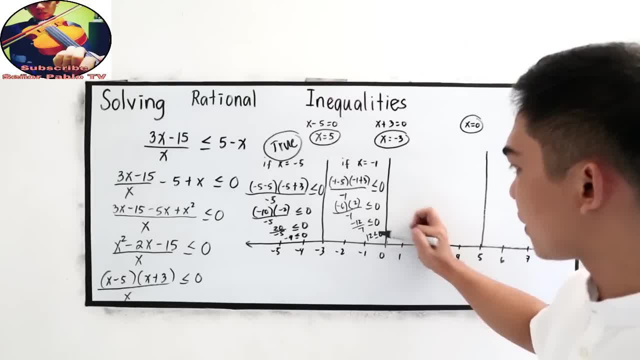 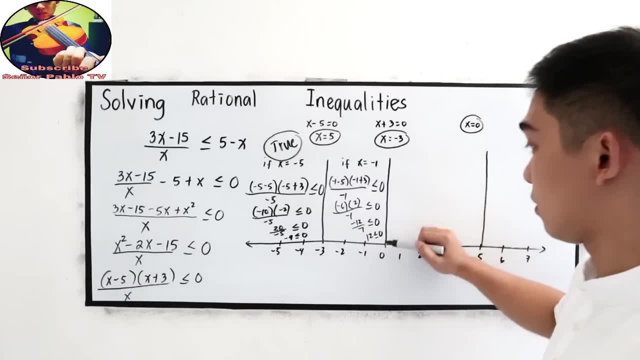 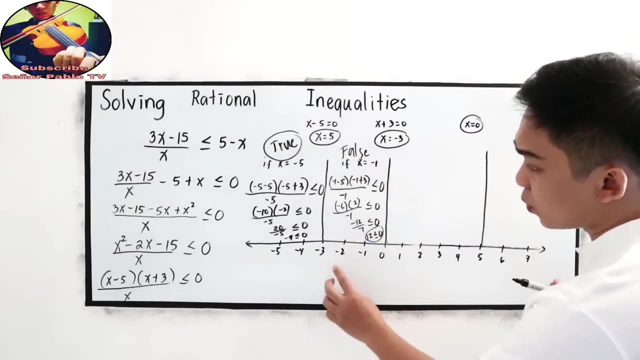 Negative 12 divided by negative 1, that is 12 less than or equal to 0.. 12 is less than 0.. True or false? False? So this is false. That means, if it is false, the numbers between negative 2 and 0 are not included. 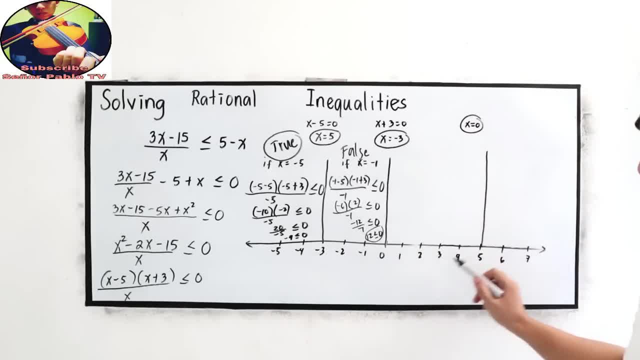 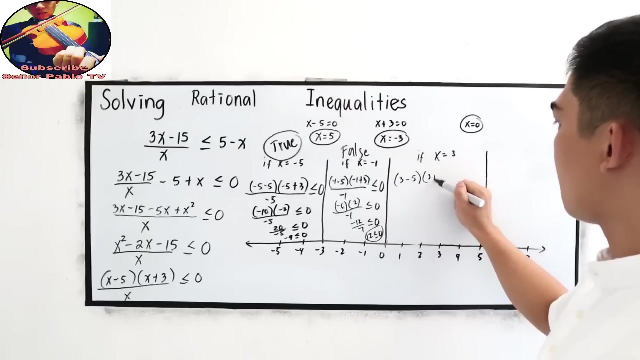 How about these numbers 1, 2, 3 and 4?? Choose 1, I will choose 3.. If x is equal to 3. So change x to 3.. So 3 minus 5, 3 plus 3 over 3 is less than or equal to 0. 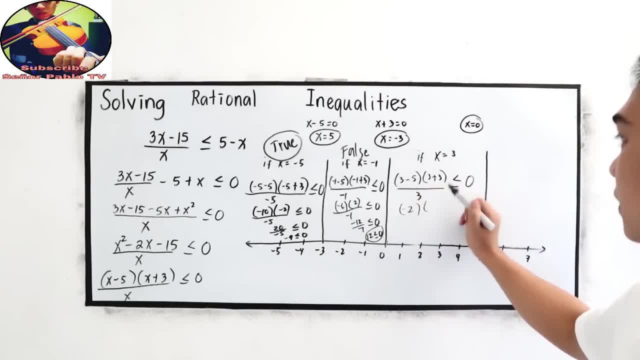 3 minus 5 is negative 2.. 3 plus 3 is 6 over 3.. Less than or equal to 0.. Let us use the cancellation method: 6 divided by 3, that is 2.. So negative 2 times 2,. this is negative. 4, is less than or equal to 0. 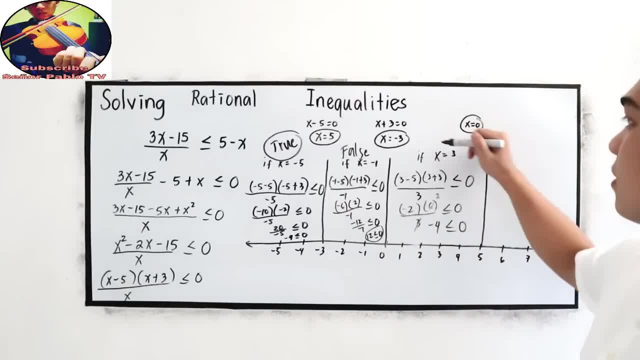 Is negative. 4 less than 0? Yes, So this is 2.. And less 6,, 7,, 8,, 9 and so on. Let us choose. if x is equal to 6.. So 6 minus 5, then 6 plus 3 over 6 is less than or equal to 0. 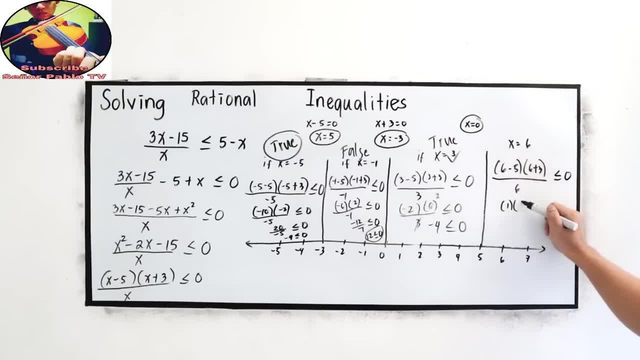 6 minus 5, that is 1.. 6 plus 3,, that is 9 over 6.. Less than or equal to 0.. So 9 over 6 is less than or equal to 0.. 9 over 6 is 1 point something. 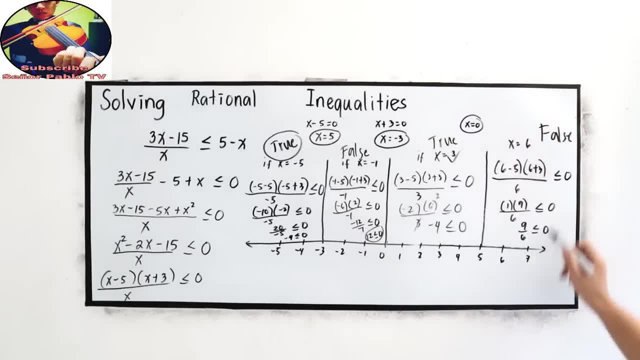 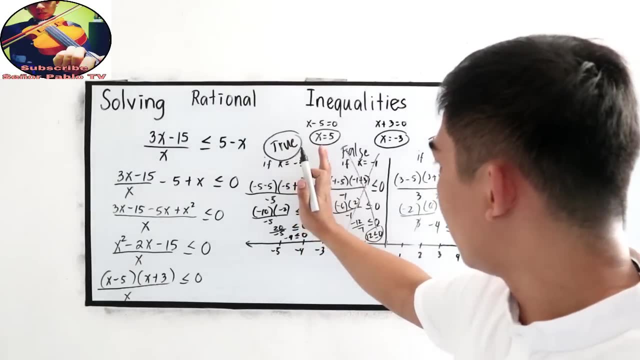 So this is false. That is 9.. Satisfies our input. So let us cross out the false And now write in our interval notation for our final answer. So in this part going to negative infinity, That satisfies our inequality.